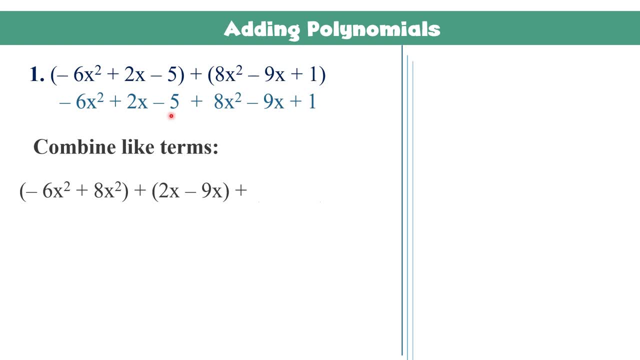 negative 5, and this one is a constant. Therefore, we may combine this to another constant term, And we have here positive 1. So negative 5 will be combined with positive 1.. Let us now add them. To proceed, you have to remember. 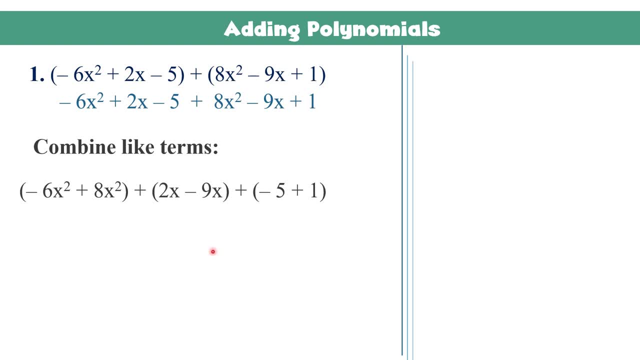 the rules in adding integers That if they have the same sign you have to add and copy the sign, But if they have different sign you have to subtract and copy the sign of the larger number. So in the first set of terms 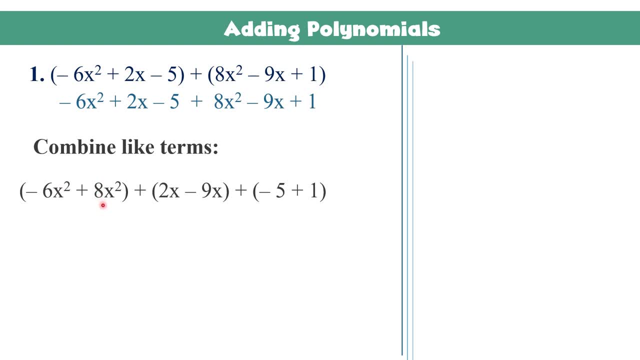 here we have negative 6 and positive 8. They have different signs, Therefore you have to subtract them. Then copy the sign of the larger number And we have positive for the larger number. Therefore your answer will be positive. So let us subtract: 8 minus 6 will have positive. 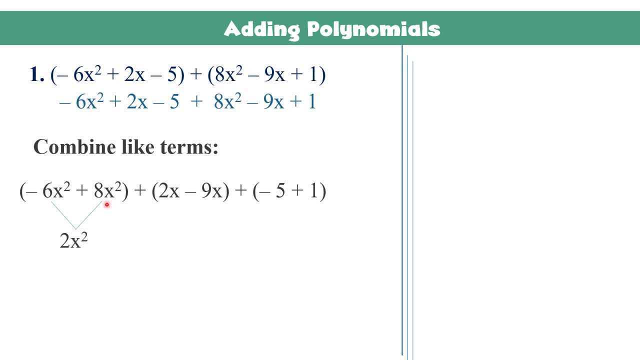 2. And then you just have to copy the variable x squared. Then let us proceed with the second set of terms, So 9 minus 9x. Again, they have different signs. So subtract and copy the sign of the larger number. 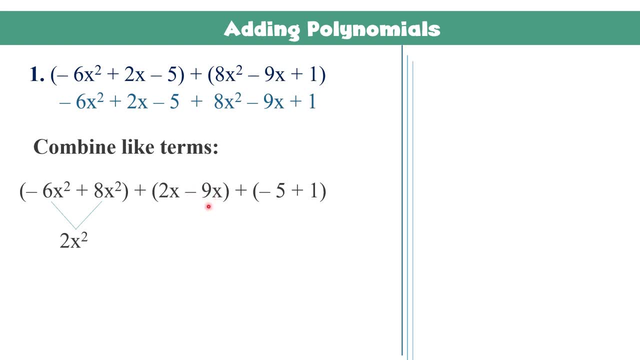 9 is larger. Therefore your answer must be negative. So 9 minus 2 will have 7.. Therefore it will become negative, 7.. And copy the variable x. Next, for the constant terms, we have negative 5 and positive 1. Different sign again. Therefore you have to subtract and copy the sign, So 9 minus. 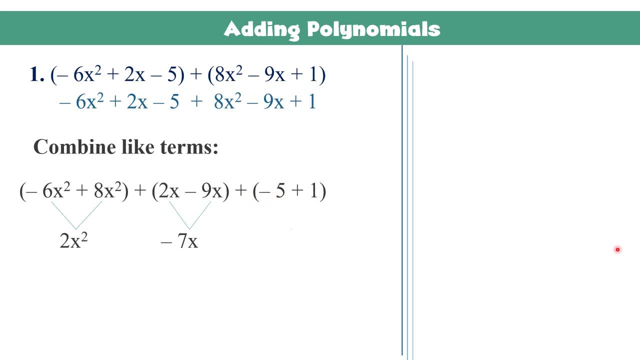 1 will give us 4. And it will become negative. Then after that, arrange it in standard form. But as you can see, they are already arranged in standard form. Therefore, that will be the answer: 2x squared minus 7x minus 4.. Aside from this method we can actually use: 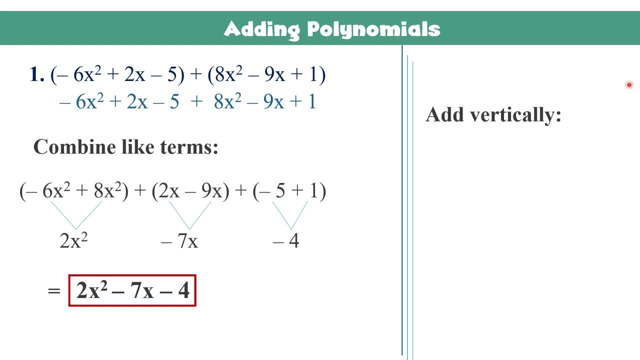 adding them vertically. So to add them vertically, just copy the first set of terms And copy the first set of terms And copy the second set of terms And copy the first polynomial. So we have negative 6x squared plus 2x minus 5.. And then in writing, the second. 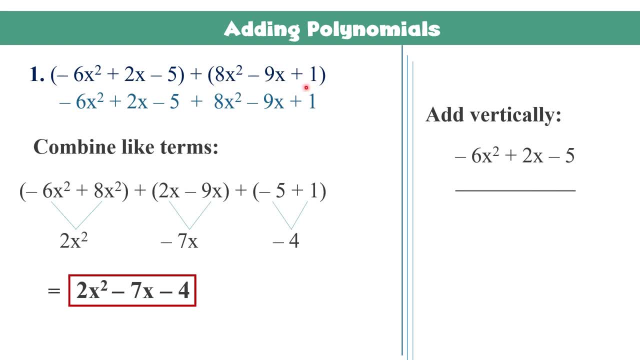 polynomial. you have to align each term here with their like terms. So it means 8x squared must be written under 6x squared, because both of them have the variable x squared. So we'll have positive 8x squared below 6x squared, Then negative 9x must be written. 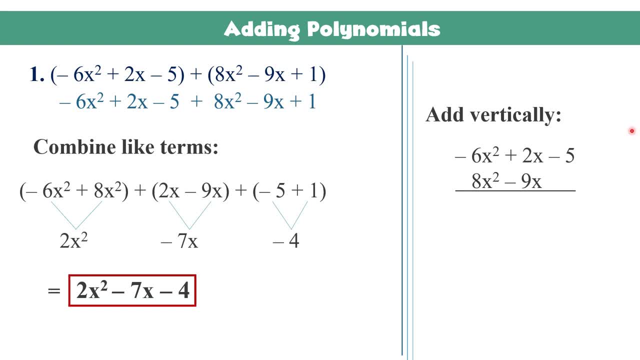 under 6x squared, So we have negative. 9x squared, So we have negative 9x squared, So we have under 2x, since both of them have the variable x, Same with the constants, So positive 1 must be. 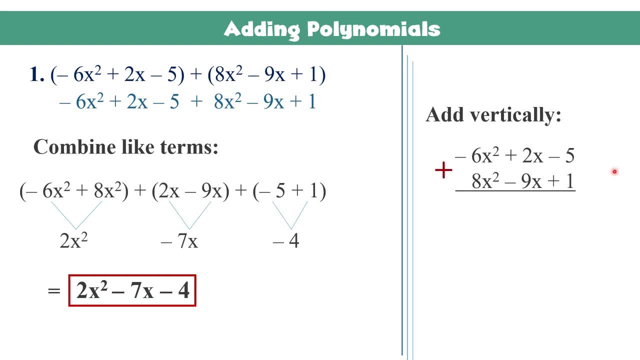 written under negative 5.. Then you may proceed with adding them. You must always remember that like terms must be aligned before you proceed. in addition, Now when you add, you can actually start from the left or from the right, It doesn't matter, You will still get the same answer. 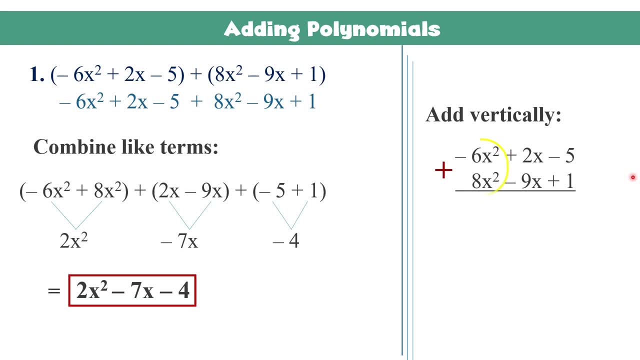 For example- I want to start here- Let us combine negative 6 and positive 8.. So negative 6 plus 8 will give us 2. And copy the variable x squared, Then the next one, positive 2 minus 9, it will. 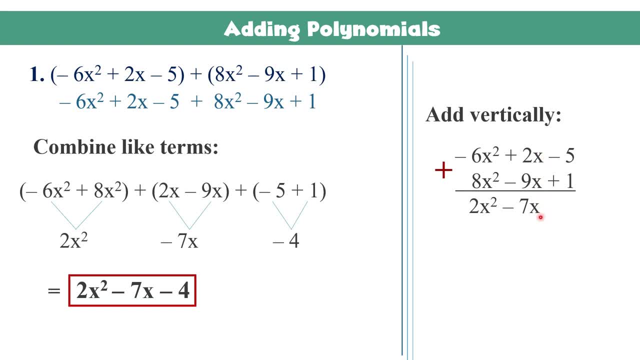 give us negative 7. Copy variable x, So we have negative 7x And for the constant term we have negative 5 plus 1. You will get negative 4. So we will obtain the same answer with this one. Whichever method is easier for you, you can use. 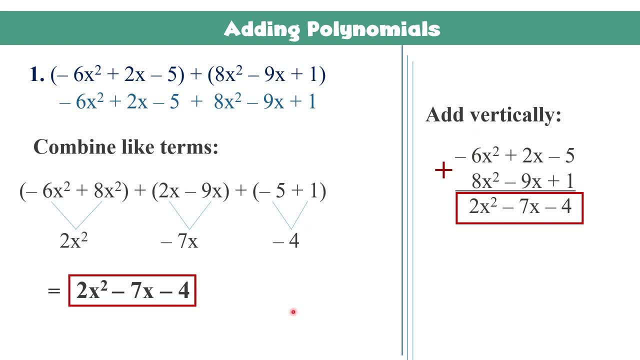 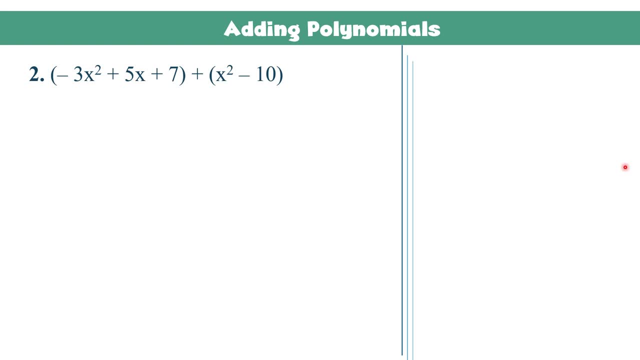 either of these two and it will give you the same answer. Another example: negative 3x squared plus 5x plus 7 plus x squared minus 10.. Again, if you will remove their parentheses, we can do that like this and then combine like terms. So let us start with the highest exponents always, so that our 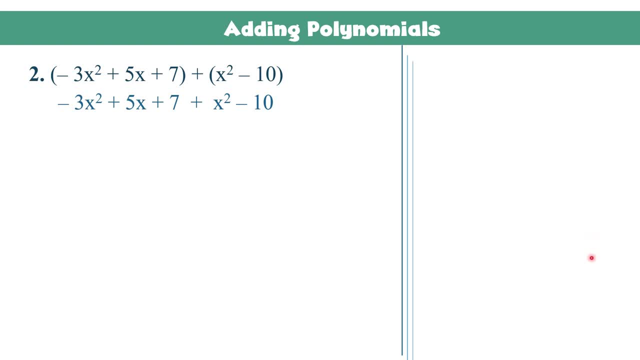 answer will automatically come out. So let's start with the highest exponents. So let's start with the highest exponents, So that our answer will automatically come out. So let's start with the be arranged in standard form. so let's start with a variable x squared. we have here negative 3x. 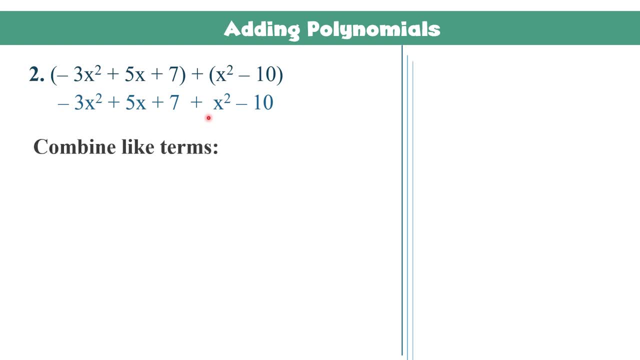 squared, and it can be combined with positive x squared here. so combine these two. we may add them directly, since they have different sign. it means we have to subtract negative 3x squared plus x squared. variable like this has always one as their numerical coefficient, though one is not. 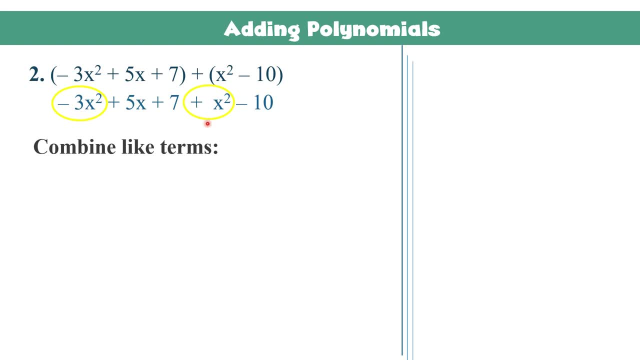 visible. so therefore we are subtracting 3 and 1, so the answer will be negative 2x squared. while it's negative, we copy the sign from the larger number, which is from 3. that's why we got negative 2x squared. then, aside from that, we have here 5x. let us look for a term with variable x. 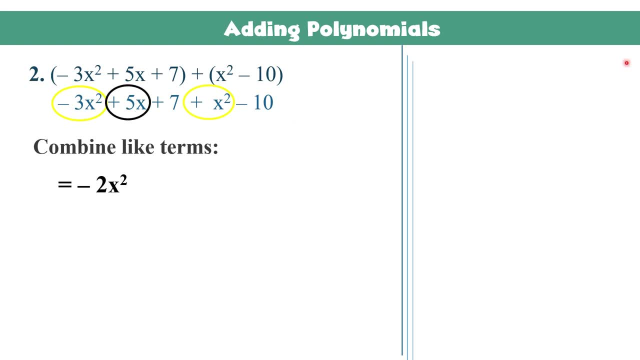 as you can see, there is no other term with the variable x. therefore we just have to bring down 5x. then for constant term, positive 7 and negative 10, again different sign. so subtract them and copy the sign from the larger number, and that's negative 10. so your answer will be negative. 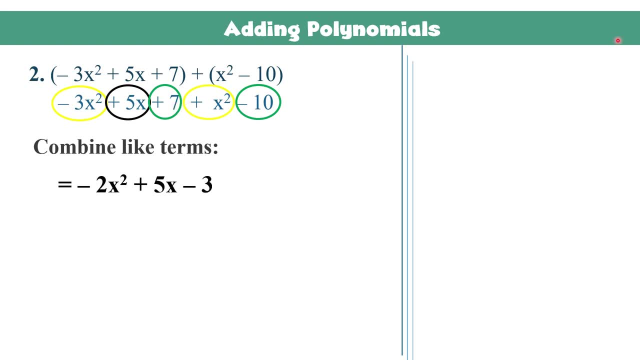 10 minus 7 will give us 3 or negative 3. so the answer is negative: 2x squared plus 5x minus 3. again, you may add that vertically copy the first polynomial and for the second polynomial you have to write each term or you have to align each term with their like term. so x squared must. 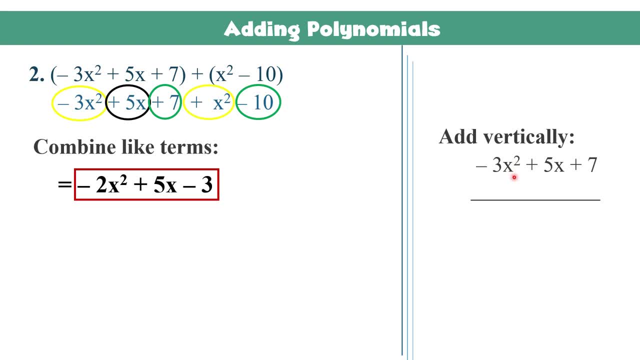 be aligned with negative 3x squared, because both of them has a variable, x squared. so negative 3x squared will have x squared below it. and then for negative 10- negative 10 is constant- we may write that under positive 7. so now let us combine them. 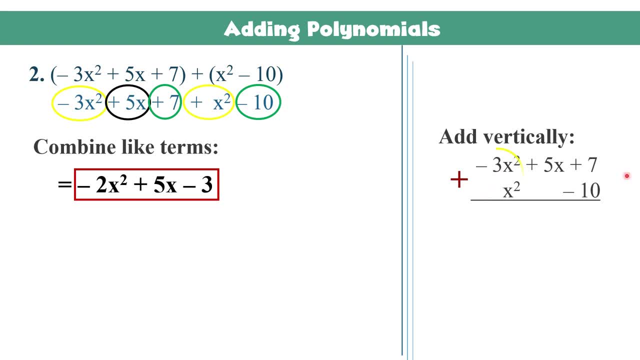 negative 3x squared plus x squared, it will give us negative 2x squared. then for 5x, actually you may just bring down 5x, then positive 7 and negative 10. positive 7 plus negative 10, it will give us, yes, that's negative 3. so this answer is the same with our answer here. 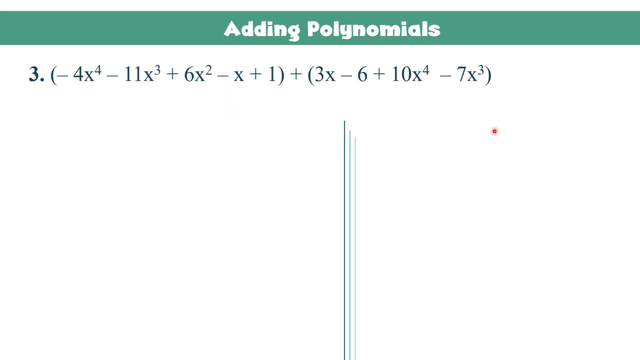 okay, another example: let us remove their parentheses and combine like terms. look for a term with the highest exponent so we can start with that highest exponent we can see here is 4, so let's start with x raised to 4. combine like terms. negative 4 x raised to 4 can be combined with positive 10 x raised to 4, since both of them. 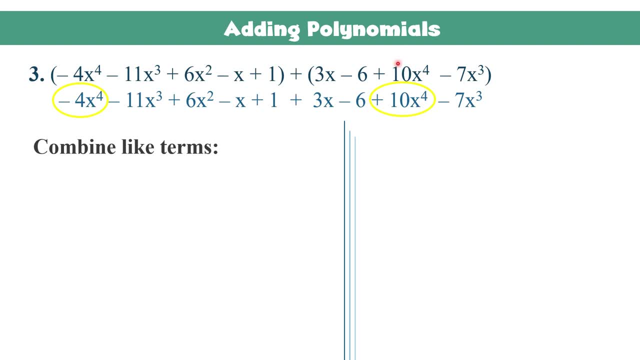 have the variable x raised to 4. negative 4 plus 10 will give us positive 6 x raised to 4. then after that we have here x cubed. negative 11 x cubed can be combined with negative 7 x cubed. so let's combine this to negative 11 plus negative 7, you will have negative. 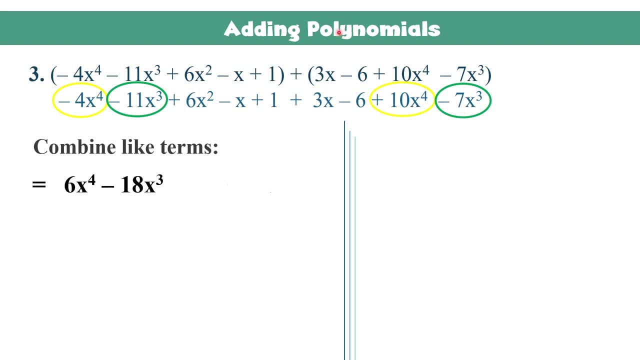 18 x cubed. both of them are negative. that's why we add the number and we copied the sign. then we have: is there any term with the variables x squared? none. so this positive 6x squared, we may just copy that. then after that we have variable x. we can combine negative x with positive 3x, so negative. 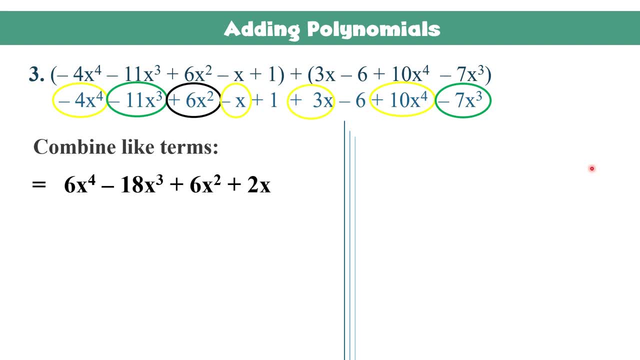 x plus positive 3x, you will have 2x, because this x has the numerical coefficient of 1, so we are subtracting 3 and 1. that's why we got 2 and we copied the sign of the larger number. then for constant we have positive 1 and negative 6. 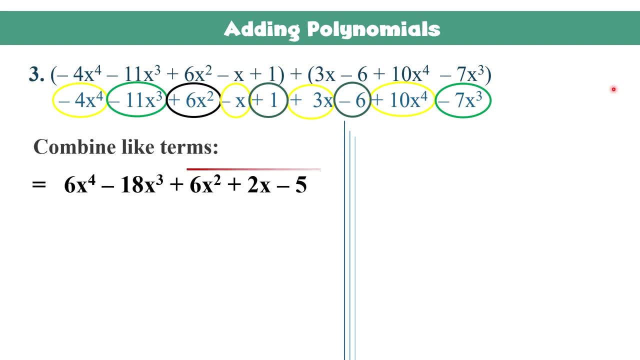 combine them you will get negative 5. so your answer is 6 x raised to 4 minus 18 x cubed, plus 6x squared, plus 2x minus 5, same with adding them vertically. copy the first polynomial and make sure to align each term from the second polynomial. 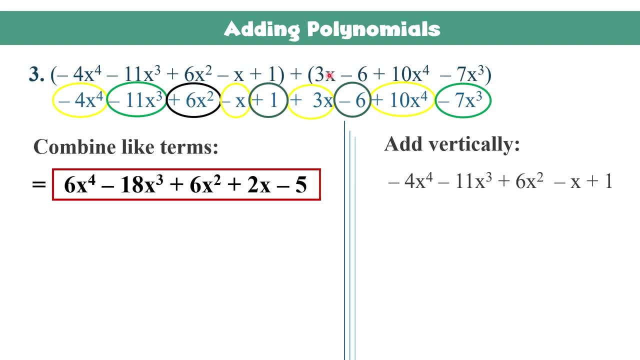 to their like terms. so let's start with 3x. so to add them you have to write this or you have to align this with its like terms. so 3x must be under negative x. negative 6 must be below positive 1. positive 10 x raised to. 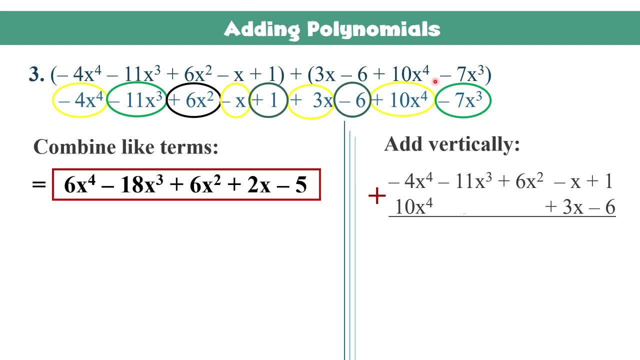 4 must be written below negative 4 x raised to 4 and negative 7 x cubed must be written below negative 11 x cubed. okay, so now we may proceed in adding them. let us combine first negative 4 and 10, you will get. 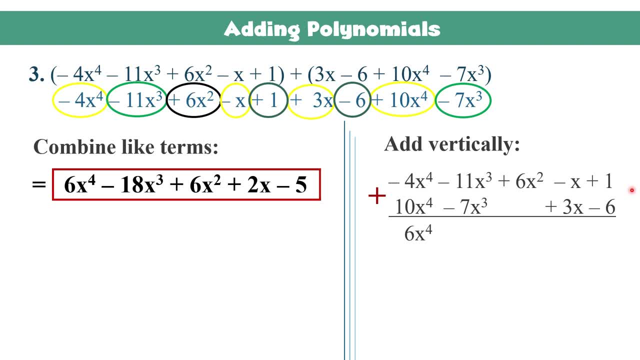 positive 6 and copy x raised to 4, then negative 11 plus negative 7. both of them are negative. that's why you have to add, and we'll get negative 18, copy x cubed, then for positive 6, x squared, since it is. 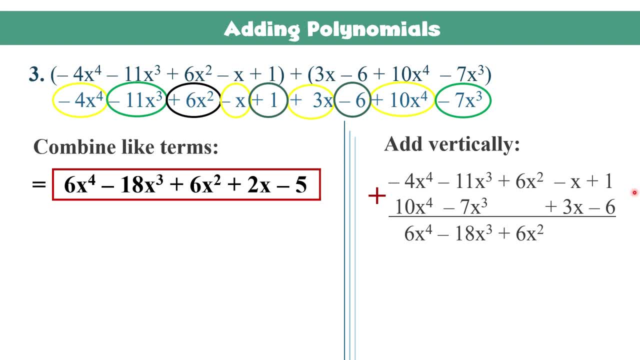 alone, you may bring the negative 6 x squared and you will get negative 6 x squared and you will get negative 3. for the positiveệu 6 x. levanting down then negative x plus 3x, you will have positive 2x and for positive, 5. so the answer is the same with: 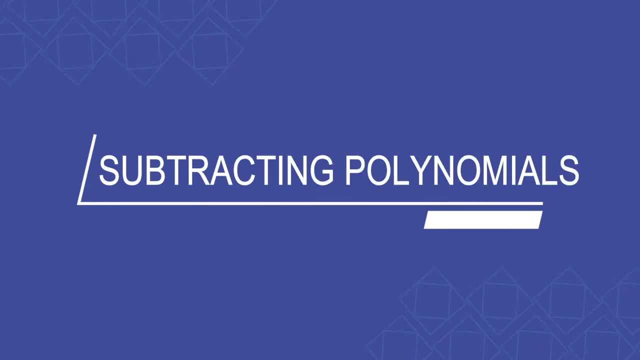 this one. the sub track polynomial is to add its inverse, so you have to switch the signs of the positive 1 x, since this is a 2 x raised to 4, respect that u have to subtract two way to add and the two おa n, 0 at, and you can form this asière- and negative 5 as share your power. 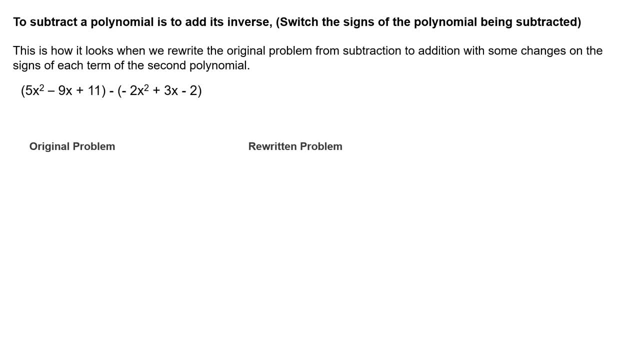 Robot networks. so keep yourusa x matrix. signs of the polynomial being subtracted or the subtrahan. Let us see in this example. the original problem is like this: 5x squared minus, 9x plus, 11 minus negative, 2x squared plus. 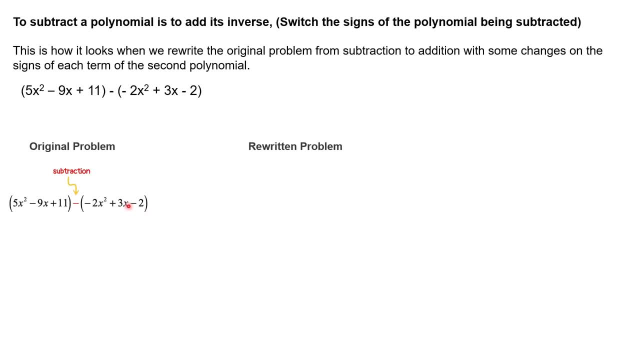 3x minus 2.. Before you proceed in solving them, this second polynomial, or the subtrahan, must be multiplied with the negative sign here or the minus sign, So it's like the sign will just be the inverse: This negative 2 became positive 2, this one and then positive 3 became negative 3. 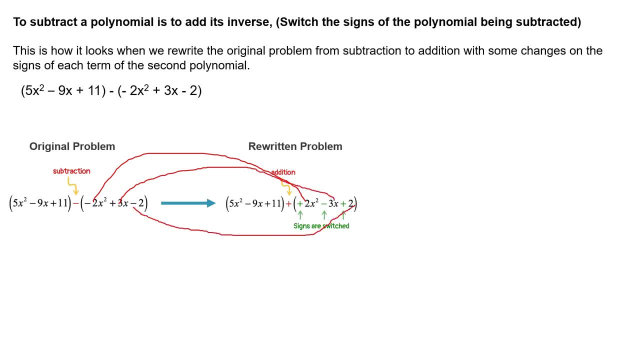 and negative, 2 here became positive. So all the signs of the second polynomial, or the subtrahan, change to its inverse, Because when we multiply negative to another, negative you will get a positive answer, Negative times positive you will get a negative answer, And negative times negative you will have. 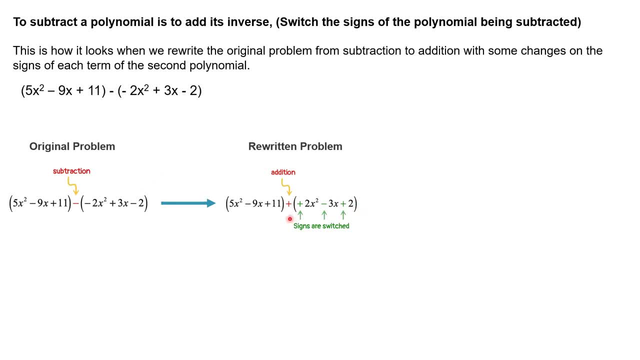 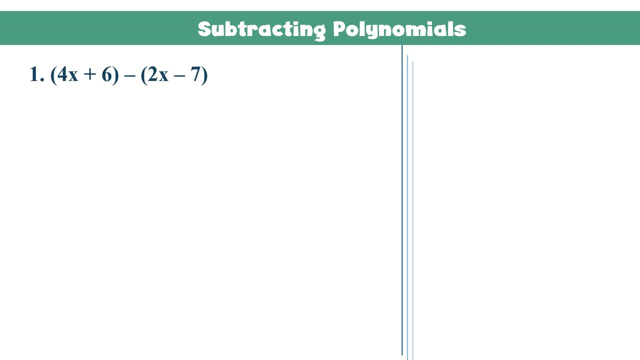 a positive answer. So you have to rewrite the problem first before you proceed in adding them. That's how we subtract polynomial. Let us have an example. For example, we have 4x plus 6 minus 2x minus 7.. 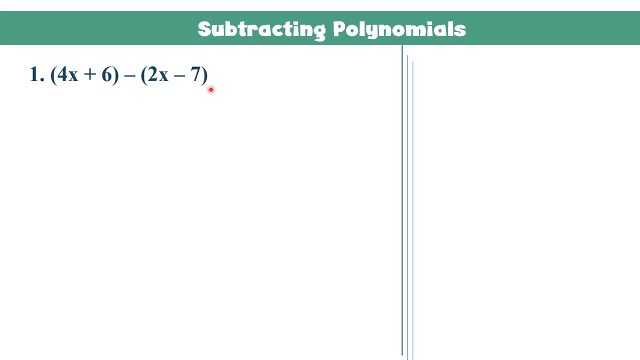 So the subtrahan here is 2x minus 7.. Before we solve, let us rewrite this problem. first Copy the first polynomial, 4x minus 6, and then multiply this minus sign or negative sign to each term inside this parenthesis. So negative times positive, you will have negative 2x and then 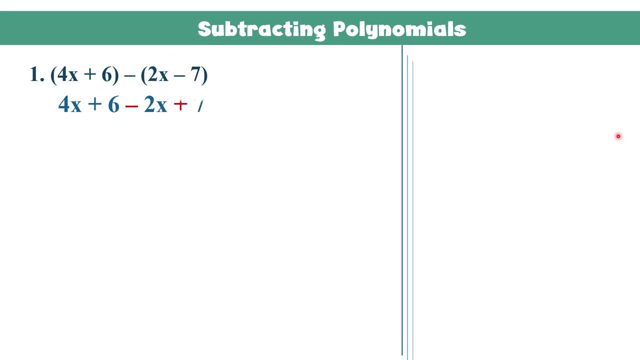 negative times: negative, negative 7, you will have positive 7.. Or in short, just change the sign of each term inside this parenthesis. So the positive 2x became negative, negative 7 became positive. Then proceed with combining like terms. 4x here can be combined with negative 2x, since both of them have the variable. 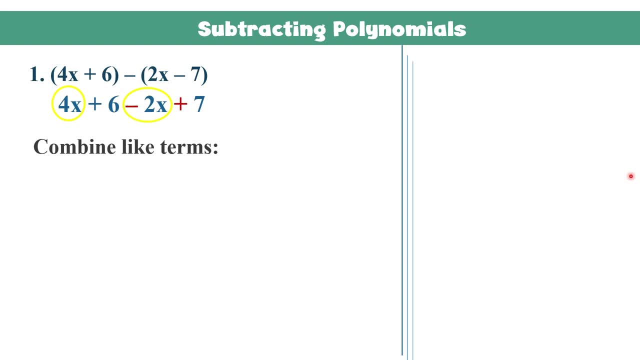 x, 4x plus negative 2x, you will have positive 2x, And then positive 6 can be combined with positive 7, you will have positive 13.. So that's it. That will be the answer In solving them. 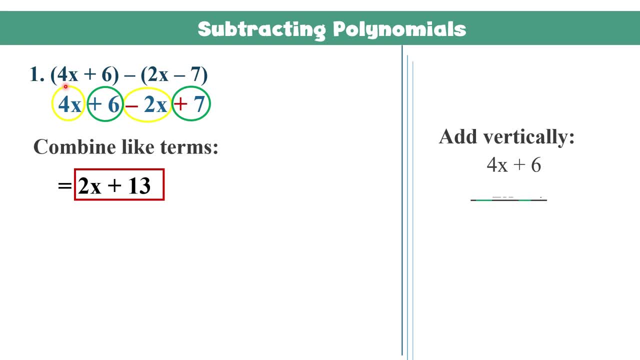 vertically you will do the same process. Copy the first polynomial, 4x plus 6. Then, before you proceed, you have to change the sign of each term inside this parenthesis, So positive 2x will be negative 2x and negative 7 will become positive, 7. Then proceed in adding them. Combine positive: 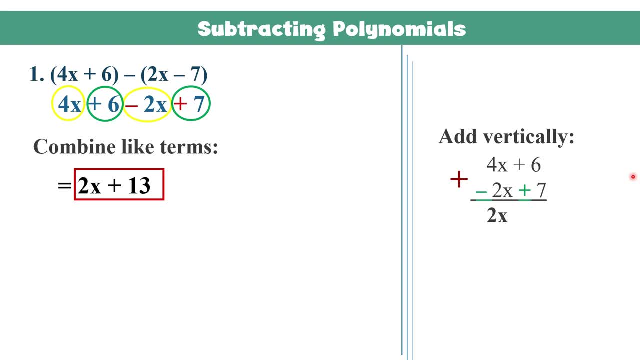 4x and negative 2x, you will have 2x, And then positive 6 and positive 7, you will have positive 13.. So the same answer with this one. Let us now proceed with the second example. So we have. 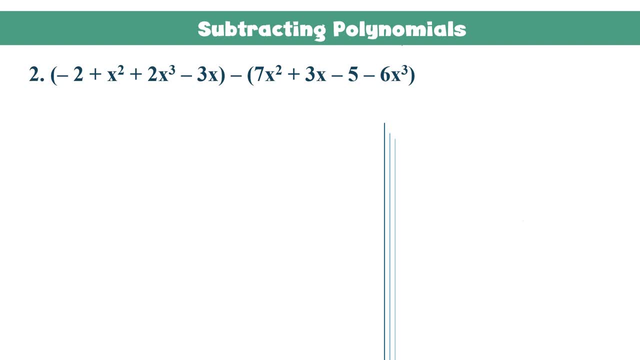 negative: 2 plus x squared plus 2x cubed. So the first step, copy the first polynomial. So we have this polynomial And then you have to change the sign of each term inside this parenthesis, or change the sign of the subtrahend. 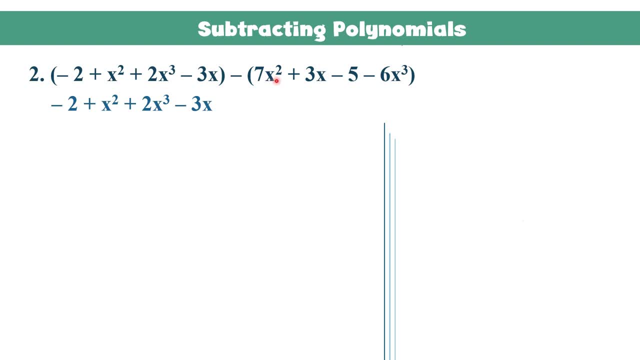 So let us start with 7x squared. 7x squared is positive, It will become negative. 7x squared Positive. 3x will become negative, 3x Negative. 5 will become positive, 5. And negative. 6x cubed will become positive 6x cubed. Now we may proceed in combining. 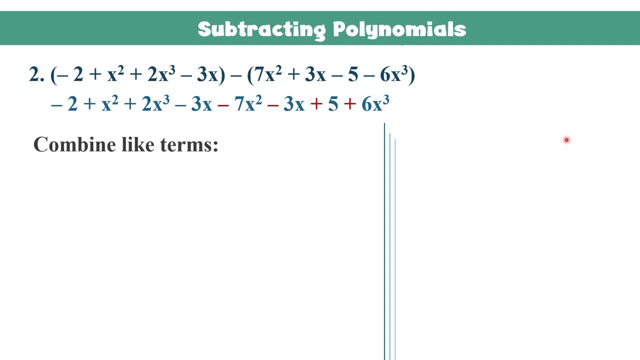 like terms And please take note that when you combine like terms, we will start with the term with the highest exponent, because we have to write our answer in standard form, So we'll start with the highest exponent. Highest exponent here is 3.. So 2x cubed and 6x cubed can be combined with. 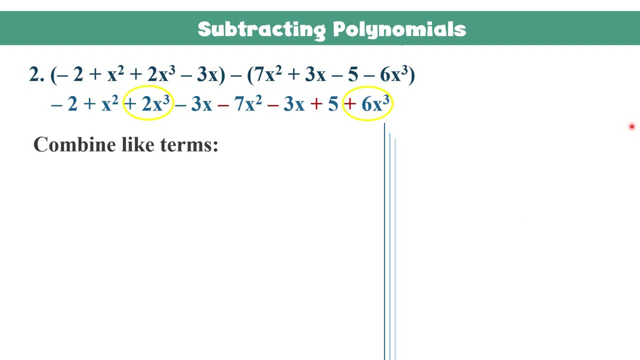 each other. They are both positive. So that will be 6 plus 2 will have 8.. And copy x cubed. Then after x cubed we have here x squared. We can combine positive x squared with negative 7x. 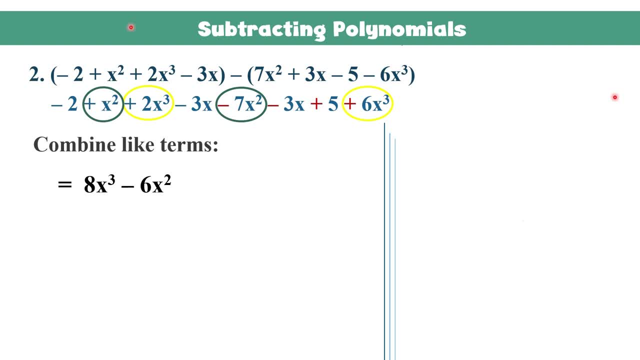 squared And you will have negative 6x cubed. Then for the term with the variable x, we have here negative 3x and another negative 3x. here We may combine these two. Both are negative, So you have to add the number and copy the sign. 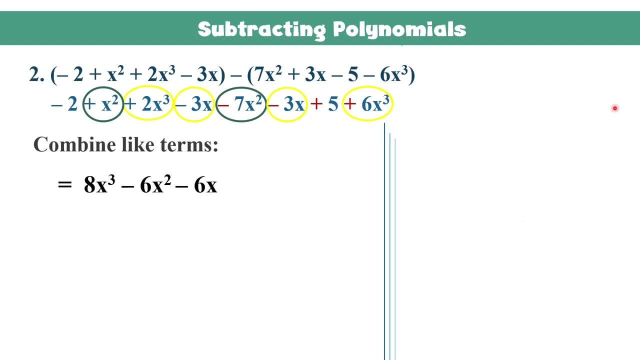 3 plus 3 will give us 6 and copy the negative sign. So we have negative 6x And for the constant terms, we have negative 2 and positive 5. Combine these two, you will have positive 3. Since they 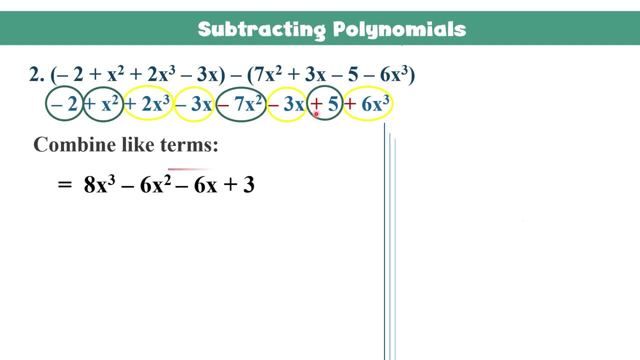 have different signs. we can combine these two And you will have positive 3. And you will have subtracted them and copy the sign of the larger number. So this one is the answer. Again, this is similar in adding them vertically, Before you start subtracting them. you have to arrange this. 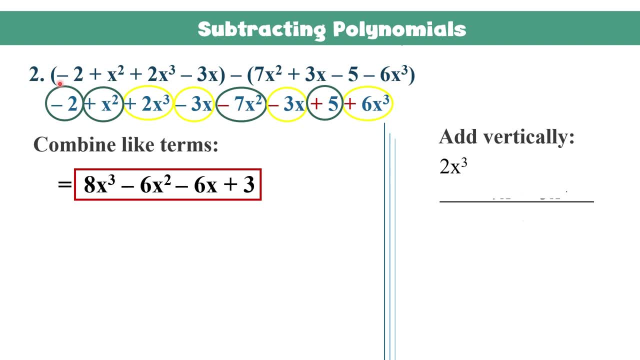 first in standard form. So let us start with the first polynomial and copy first the term with the highest exponent. So we have here positive 2x cubed, So positive 2x cubed, And then after that we have here positive x squared. We may write positive x squared. 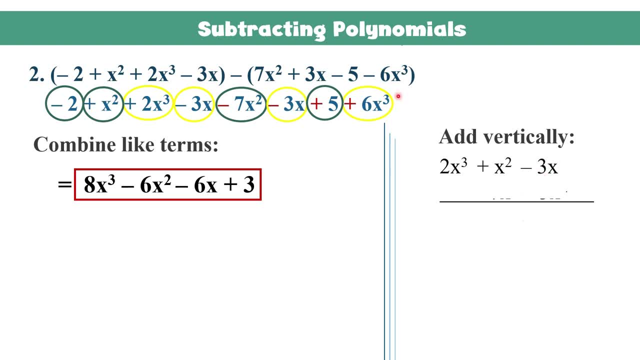 Then after that, negative 3x, Negative 3x here and negative: 2.. Then align the second polynomial. But please take note, you have to change the sign while you are copying it. So let us start with 7x squared. 7x squared positive. It will become negative And you will write that under x squared. 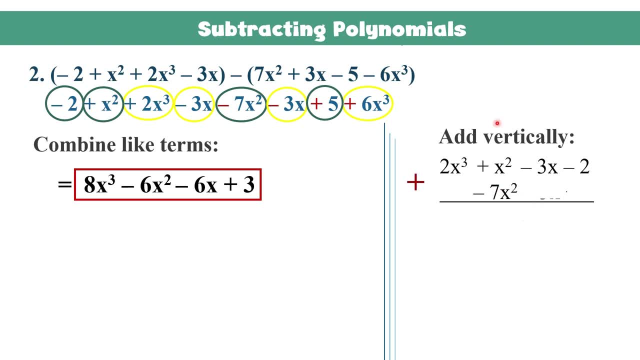 because they have the same variable. Then after that we have positive 3 here, Change the sign, It will become negative And you will write that under x squared because they have the same variable. Negative 3x And write it under negative 3x, Then constant term: negative 5 will become. 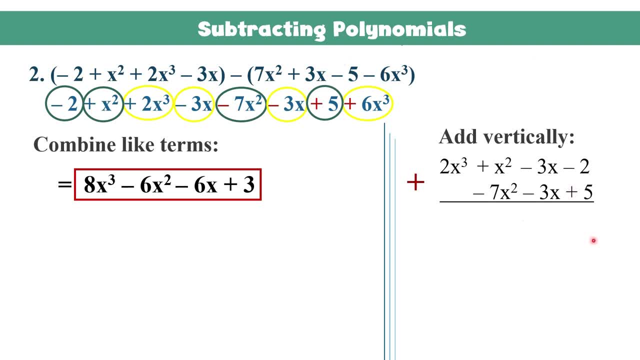 positive 5.. Write it under negative: 2. While the last term here negative, 6x cubed. So x cubed it means it must be under 2x cubed. It is negative, So therefore you will change it into: 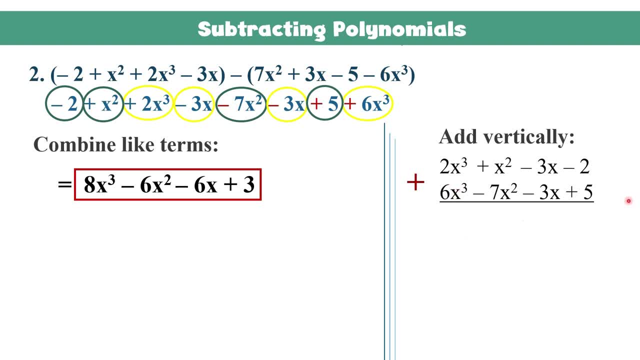 positive, Then combine. You may start from left or from right, It does not matter. So let us add first this side, 2 plus 6, you will have 8.. Copy x cubed, Then positive x plus negative 7. So they have different sign. You have to subtract And you will get negative 6x squared. 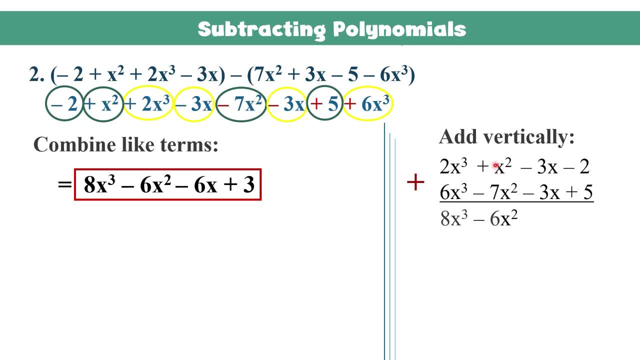 because x squared has the coefficient of 1 that we do not see, And then negative 3x plus negative 3x. Both of them are negative. You have to add them, So you will have negative 3x plus negative 6x And negative 2 plus 5, different sign. So you have to subtract. You will get positive 3.. 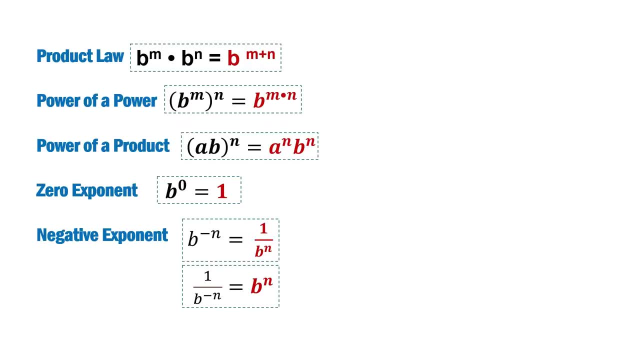 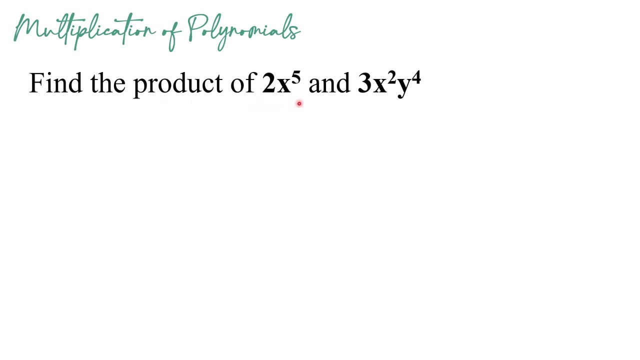 So the answer is similar to this one. In multiplying polynomials, you must have the knowledge of these laws of exponents. Let us proceed with the examples. First, find the product of 2x raised to 5 and 3x squared y raised to 4.. 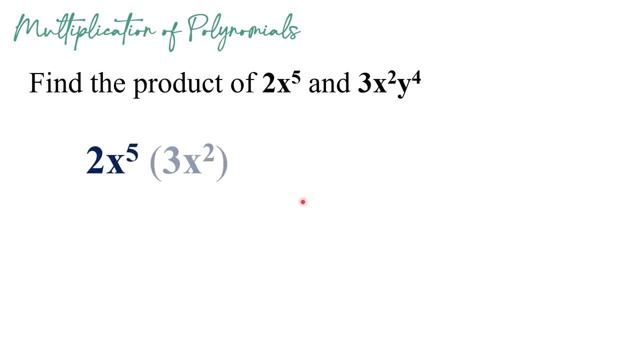 To multiply this 2, let us start with the numerical coefficient 2 times 3.. 2 times 3 will give us positive 6.. Then proceed with the variable, So multiplying x raised to 5 and x squared. Since they have the same base, which is x, then we just have to add their exponent, So it will be 5 plus. 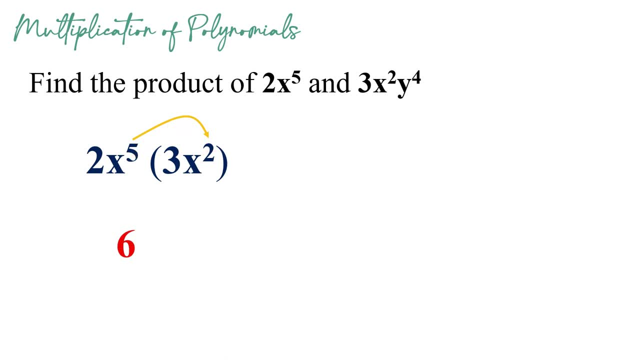 2. And it will give us 7.. So we have 6x raised to 7.. Then our final answer is 6x raised to 7.. Another example: Let us find the product of 5m and m squared plus 9.. So to write that: 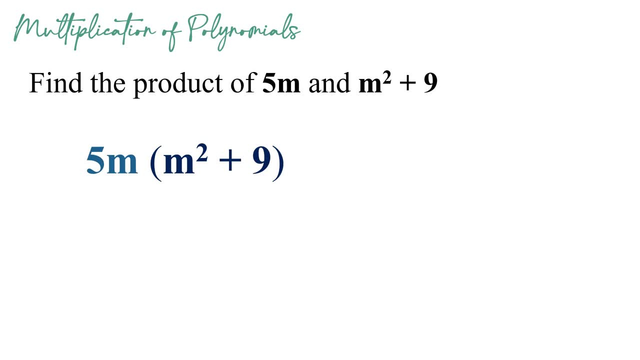 we'll have 5m outside and m squared plus 9 inside the parentheses, since they are together. To multiply this monomial to a binomial, we have to distribute 5m to each term inside this parentheses. Let us start with 5m times m squared, Since m squared has no numerical. 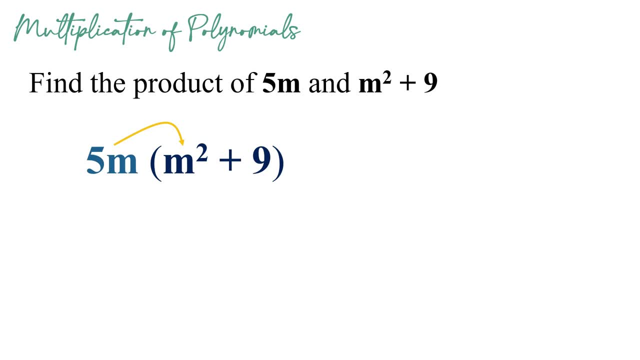 coefficient. it means we just have to multiply their variable. So m times m squared. This m- since you do not see the exponent automatic, it is 1. So it's like we are adding 1 plus 2.. Therefore, 5m multiplied to m squared will give us: 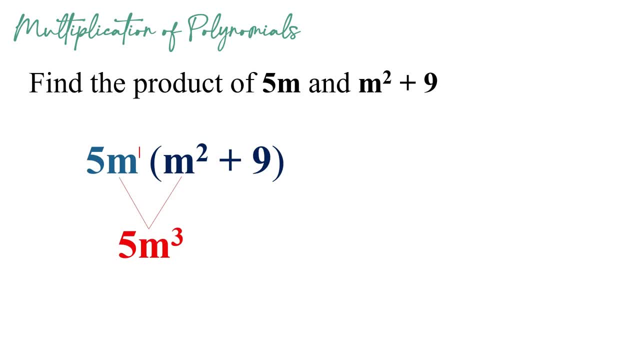 5m raised to 3 or m cubed, So we had 1 plus 2. It became m cubed. Then for the other term, let's multiply 5m to 9.. Since 9 has no variable, it means we just have to multiply 5 and 9. Then 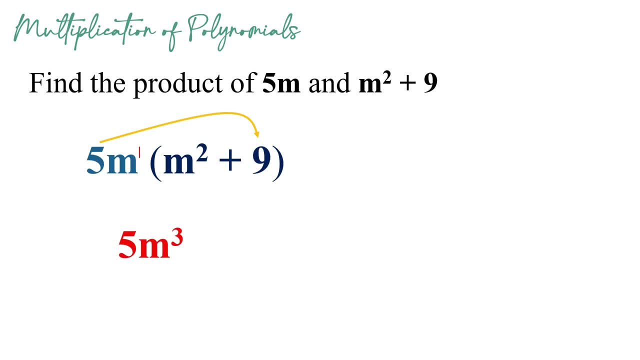 copy the variable m. So 5 times 9 will give us positive 45. Then just copy the variable m. So that's it. That will be our answer. Next example: Let us find the product of 3a squared and 2a cubed minus 5a plus ab. So we have 3a squared times 2a cubed minus 5a plus ab. What we 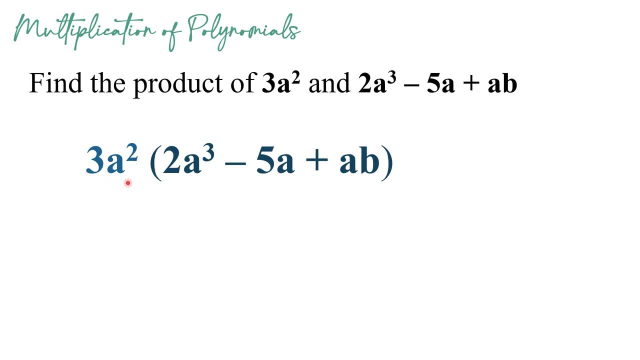 have to do here is to multiply this monomial to each term inside this parentheses. So multiply it to 2a cubed. After that 2 negative 5a squared. So we have 2a squared times 2a cubed, minus 5a plus ab. 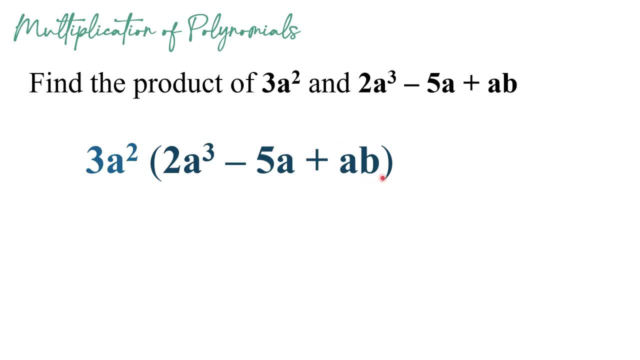 And then to positive ab. Let's start with the first term of this trinomial, Multiplying 3a squared times 2a cubed. we have to start with their numerical coefficient, 3 and 2. It will give us positive 6. Then for their variables, since they have the same base, then it means we: 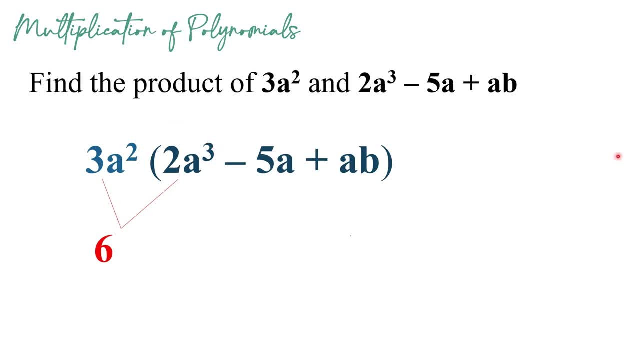 just have to add their exponent. So 2 plus 3 will give us 5.. So we have here 6a raised to 5.. Then for the second term of this trinomial, let's multiply it with 3a squared, 3a squared. 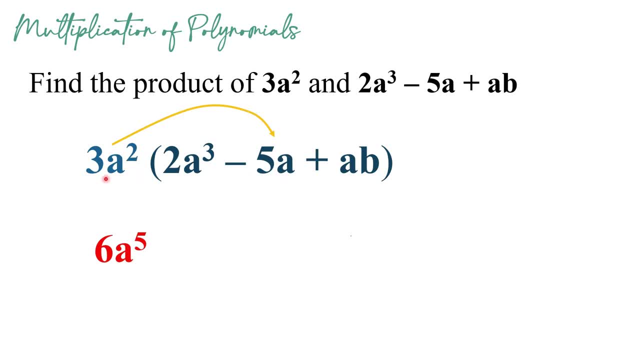 times negative 5a. So multiply first their numerical coefficient 3 times negative 5. It will give us negative 15.. Then for their variable, a squared times a, you will have a cubed, Since the exponent of this a is 1. So it's 1 plus 2.. 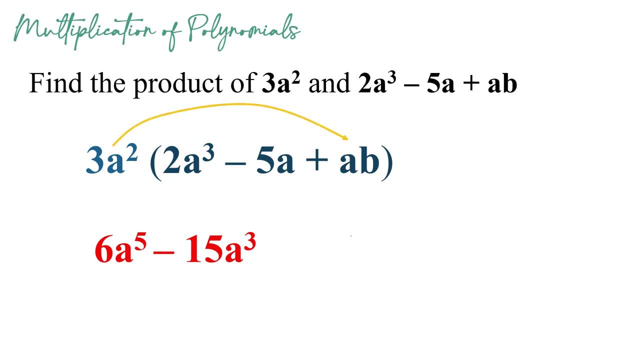 It will give us 3.. Then for the last term, 3a squared times ab. Since it has no numerical coefficient, we'll just copy 3.. And let's multiply their variable. So we have a squared here and a again It means raised to 1.. So we'll be adding 2 plus 1.. Then variable b: we just have to copy it. 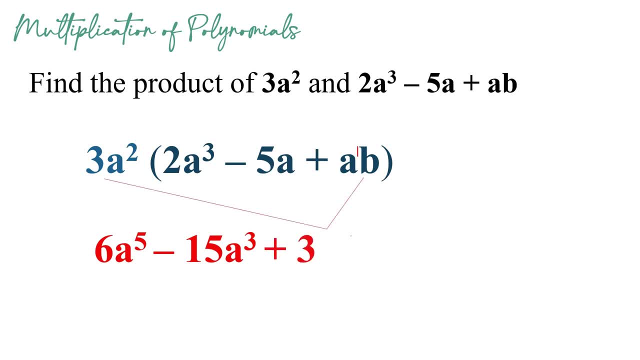 So 2 plus 1 will give us 3.. So therefore it will become 3a cubed, Then just copy b. So this is the final answer. Let us have more examples. Find the product of 4x plus 5 and 3x minus 7.. As you can see, 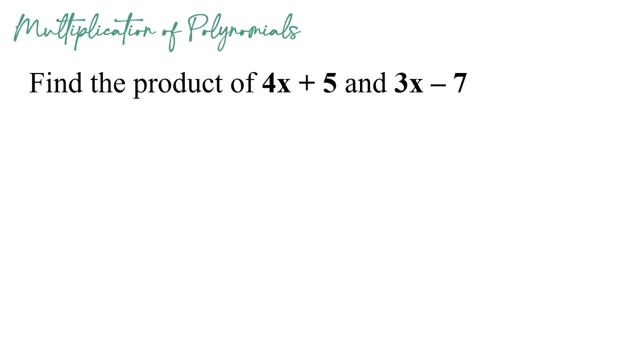 the polynomials we have here are both binomial. So when you multiply binomials, it will be like this, And the method that we are going to use in multiplying them will be the FOIL method. So what does FOIL method mean? 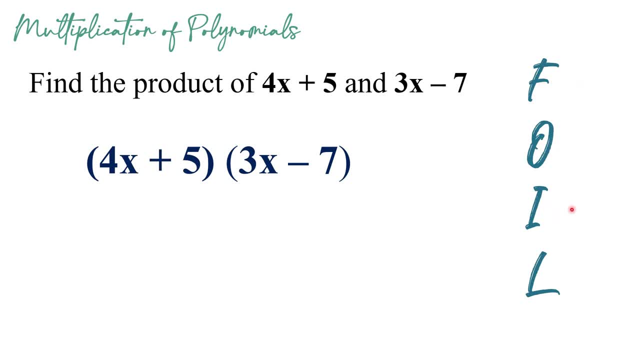 FOIL means first terms: O for outer terms, I for inner terms and L for last terms. So for F we have to start with the first terms. It means that is the first term of each binomial. So for the first binomial the first term is 4x, And for the second binomial the first term is 3x. So we 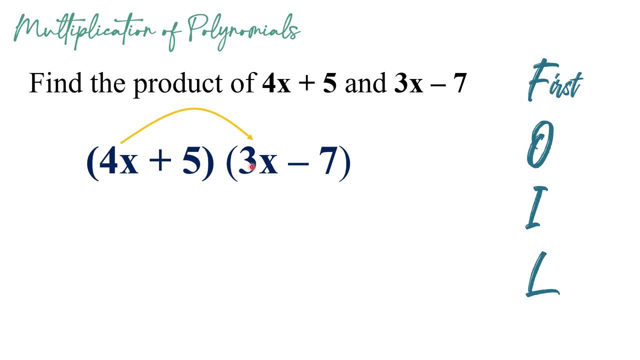 have to multiply them first. 4 times 3 will give us 12.. And then x times x will give us x squared. Since they are both raised to 1, we have to multiply them first. So we have to multiply them raised to 1.. Then, after that, after multiplying the first terms, we will proceed with O. 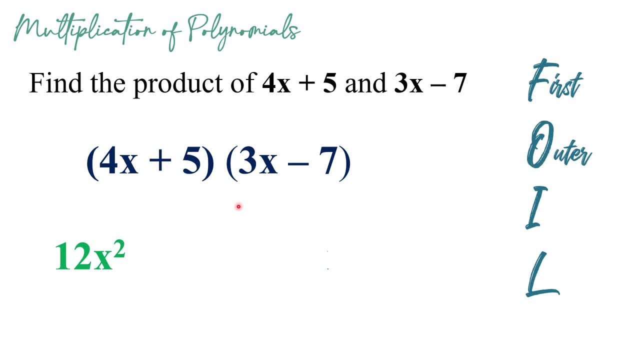 which means the outer terms. So the outer terms of these two binomials are 4x and negative 7.. 4 times negative 7 will give us negative 28.. And then just copy the variable x After O. let's proceed with I. It means inner terms. Let us multiply the inner part of the. 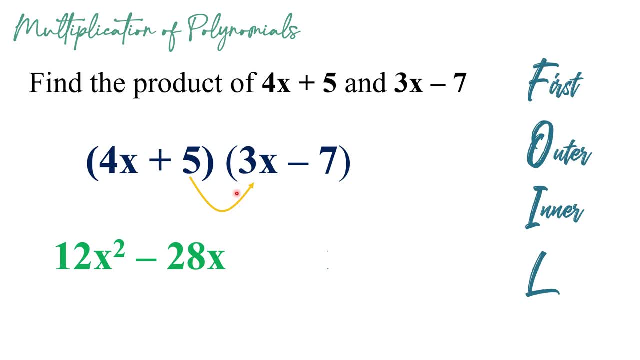 binomial. So we have 5 times 3x. 5 times 3 will give us 15.. And just copy the variable x. Then for the last letter, L, which means last terms. So we will multiply the last term of this. 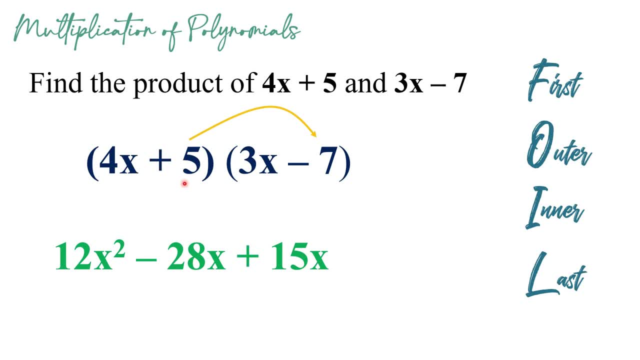 binomial: 5 times negative 7.. 5 times negative 7 will give us negative 35.. But we are not yet done. Observe this polynomial. We can still combine some of these terms, which we call the like terms. So, as you can see, negative 28x and positive 15x, they have the same variables. 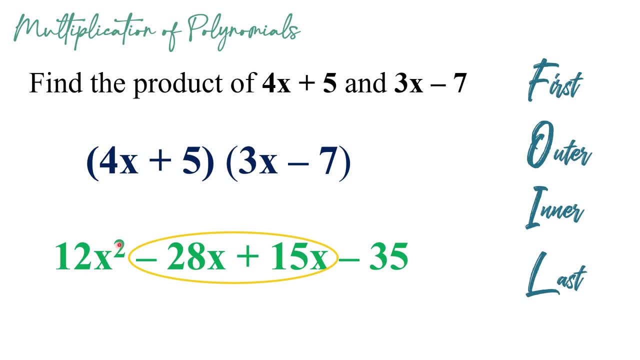 And therefore we may combine them: 12x squared and negative 35,. since they do not have like terms, we may just bring down these two terms and combine these two Negative 28x plus 15x. they have different signs, So you have to subtract and copy the. 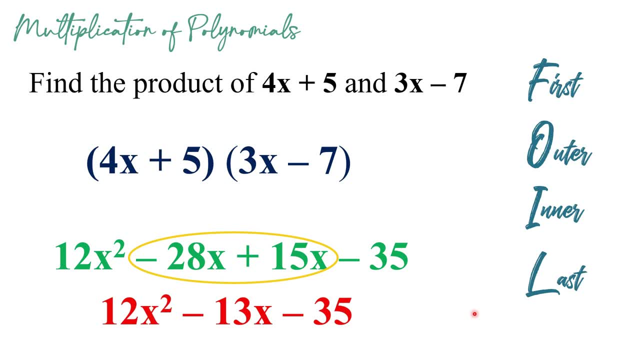 time from the larger number, The answer will be negative 13.. Then bring down x, So the final answer is 12x squared minus 13x minus 35.. But what if we have to find the product of 2x plus 5,? 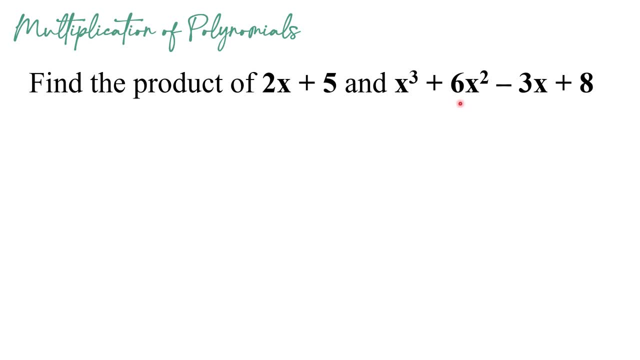 that is a binomial. and x cubed plus 6x squared, minus 3x plus 8, that is a multinomial. So how are we going to multiply them? To do that, we will start by multiplying them. So we will start by: 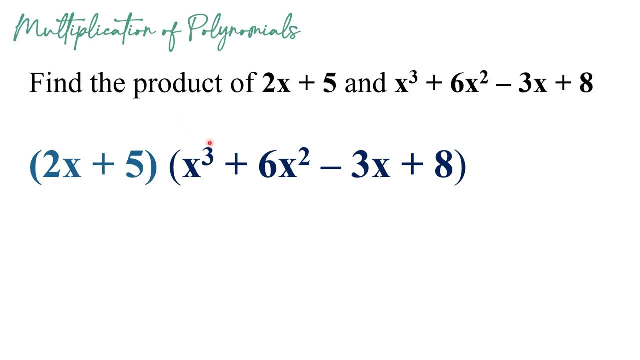 multiplying them to each term of this multinomial. Then after that, we will proceed to the second term, which is the positive 5, and multiply this again to each term of this multinomial. So let's start with the first term: 2x, Multiply 2x and x cubed So to multiply them. 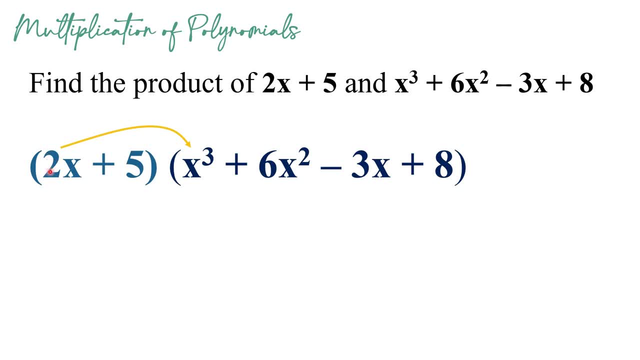 you just have to bring down or copy the numerical coefficient, then multiply their variables. So we times x cubed, It will give us 2x raised to 4, since the exponent of this x is positive 1.. So we just added 1 and 3. We got 4.. Then next 2x times 6x, squared, Just multiply first their. 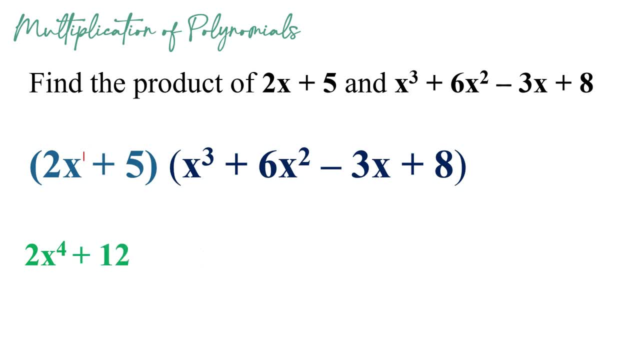 numerical coefficient 2 times 6 will give us 12.. Then after that multiply their variable x and x squared will give us x cubed, since we will add 1 and 2.. Then next, 2x times negative, 3x, We have. 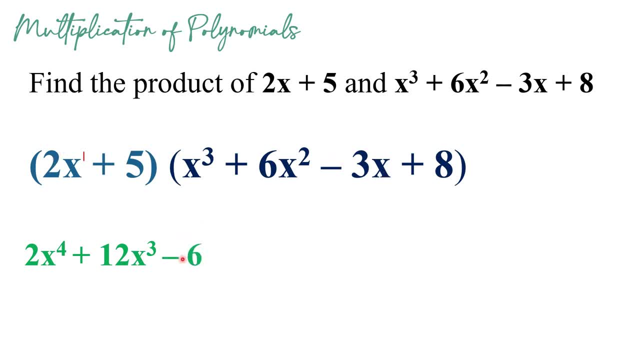 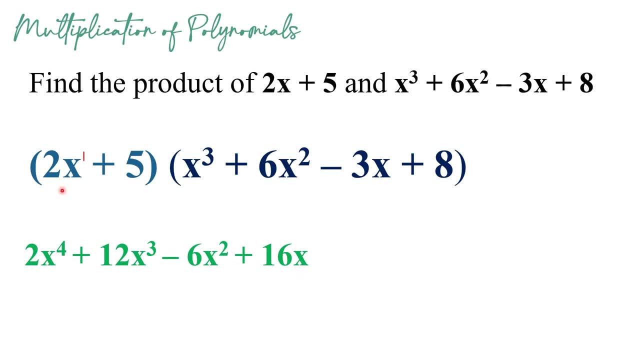 x, So positive 16x. Since we're done with 2x, let's proceed with the second term, 5, and multiply this to each term of this multinomial. Let's start with 5 times x cubed. 5 times x cubed will have: 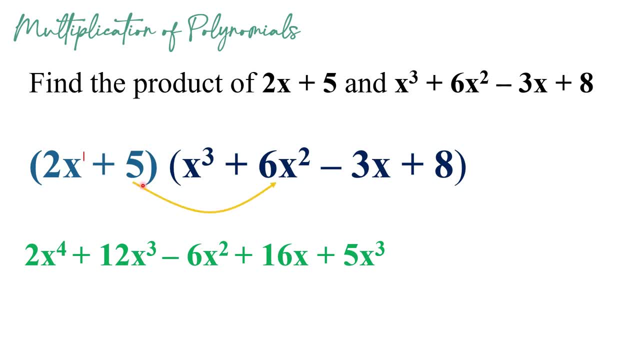 positive 5x cubed. Then 5 times 6x squared, Multiply 5 and 6.. We'll have positive 30.. And just copy the variable x squared. And then 5 times 6x squared, Multiply 5 and 6.. We'll have positive 30.. And just copy the variable x squared. 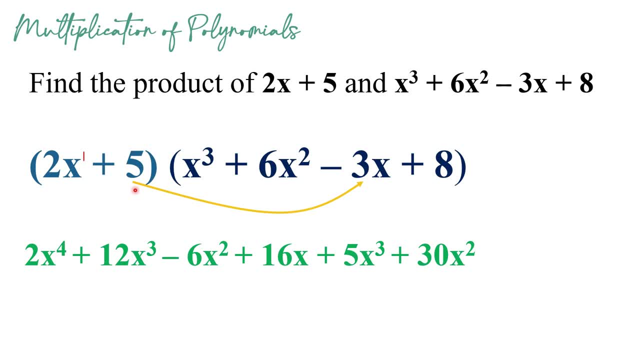 Then 5 times negative 3x, 5 times negative 3 will give us negative 15.. Then just copy the variable x, So negative 15x, And for their last terms, 5 times positive 8.. Both are positive, So your answer. 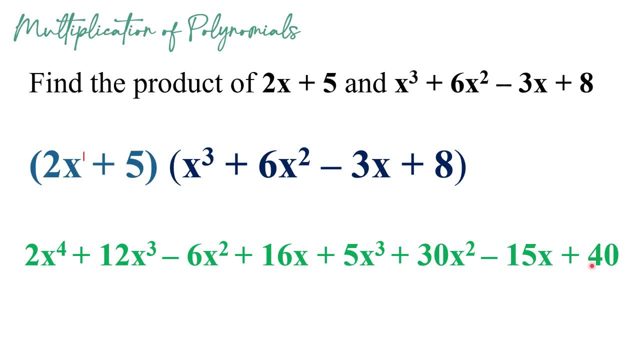 will just be positive. 5 times 8 will give us positive 40. But we are not yet done. Observe, We can actually simplify this polynomial by combining their like terms. So let's start with the first term: 2x raised to 4.. Does it have like? 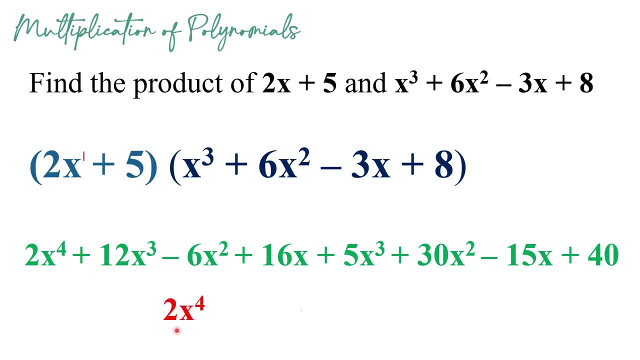 term None. So therefore we may just bring down 2x raised to 4.. Then proceed with the next term, 12x cubed. We can actually combine it with positive 5x cubed, since both of them have. 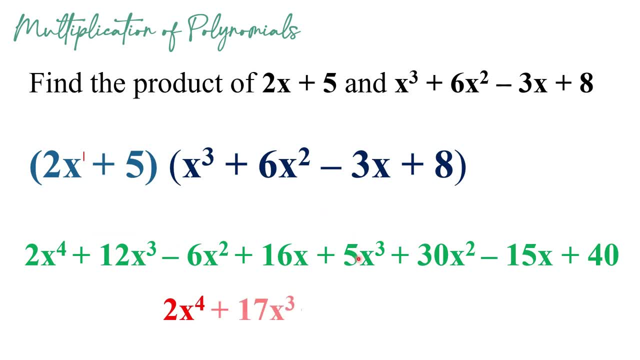 the variable x cubed, 12 plus 5 will give us 17.. Copy the variable x squared So we have the variable x cubed And then negative 6x squared. Combine it with positive 30x squared, Negative 6 plus 30. They have different signs, So you have to subtract. 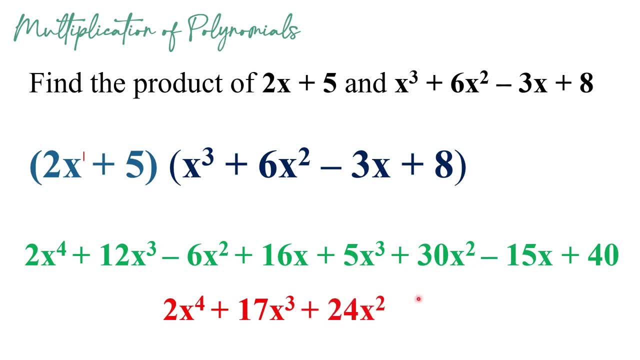 You will have positive 24.. Then copy the variable x squared, Then after that positive 16x, combine it with negative 15x. since both have the variable x 16 plus negative 15, you will actually get positive 1. then just copy the variable x, but we will only 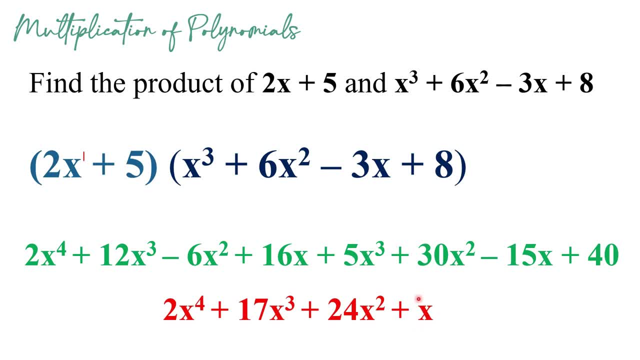 write positive x, since if the numerical coefficient of a variable is 1, we do not have to write that. so we'll have here positive x and for the last term positive 40. it doesn't have like term, therefore we will just bring down positive 40. so the answer is 2x raised to 4 plus 17x cubed plus. 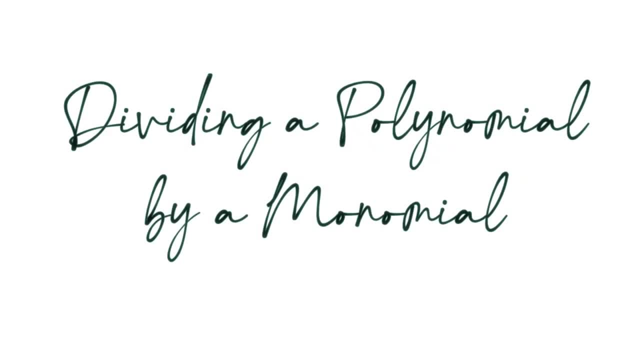 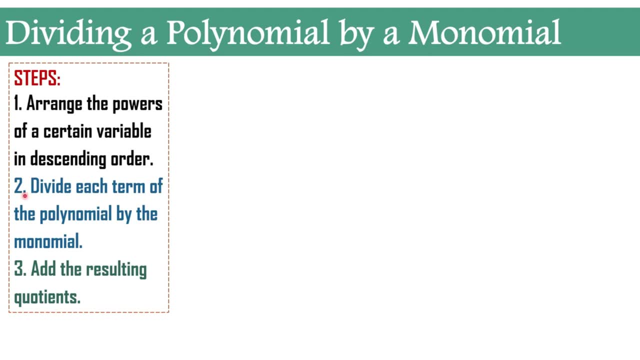 24x squared plus x plus 40. dividing a polynomial by a monomial. here are the steps on how to divide a polynomial by a monomial. first arrange the powers of a certain variable in descending order, so that your final answer will be in standard form, and then divide each term of the polynomial. 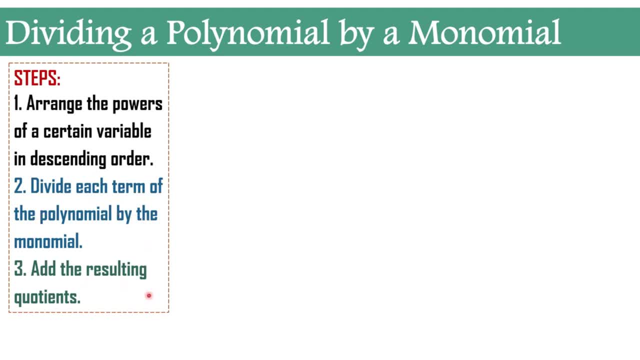 by a monomial, so that your final answer will be in standard form, and then divide each term of the polynomial by a monomial, so that your final answer will be in standard form, and then divide each term of the polynomial. after that, add the resulting quotients. for example, we have here negative 15x plus 35x, cubed plus 50x. 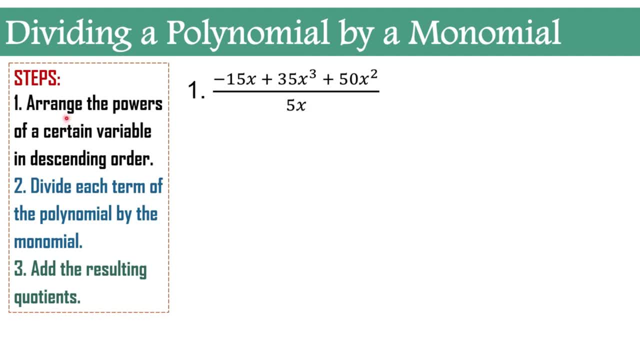 squared over 5x. first step is we have to arrange the powers in descending order. so here, the highest exponent we have is cubed, followed by squared and then raised to one. so if we do not see the exponent, it means that's raised to one. so when we arrange it will become 35x cubed, followed by positive 50x squared, and then 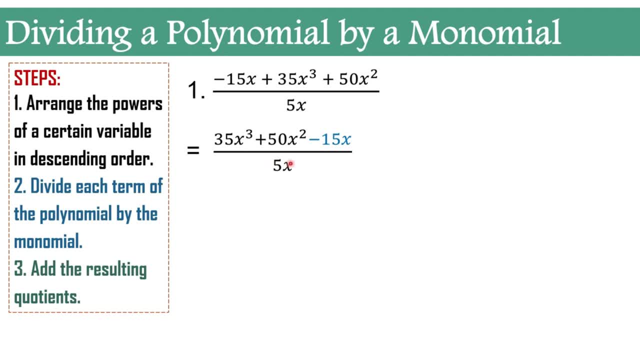 negative 15x, all over 5x. 5x is our divisor. so after that, after you arrange the powers, you may now proceed with the second step: divide each term of the polynomial by the monomial. so it will become like this: each term and the numerator will have the denominator of 5x. 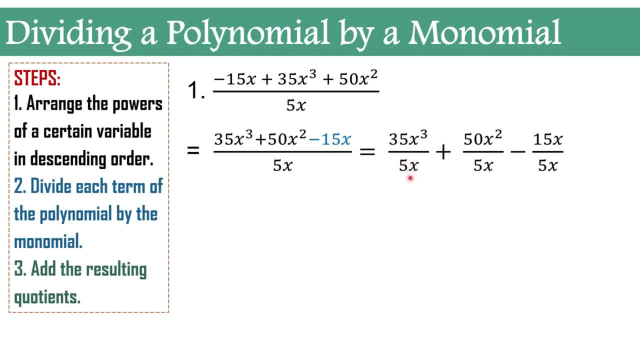 we will be dividing each term by the monomial 5x. so let's start here. you may divide first the numerical coefficient 35 and 5. so 35 divided by 5, you will have 7, followed by the variable. in dividing variable, you just have to subtract their exponent, so it will be 3 minus 1, you'll have. 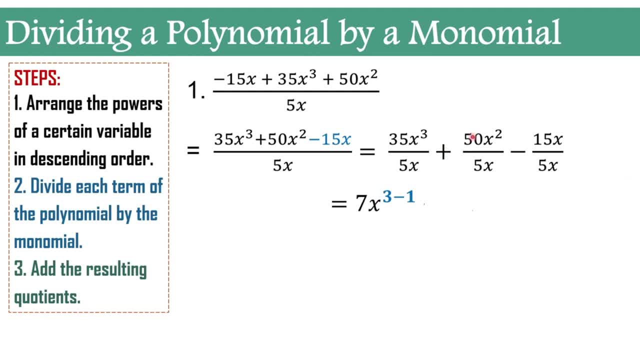 x raised to 3 minus 1, then second term, we have 50 divided by 5. so 50 divided by 5, you will have positive 10 and then x squared divided by x. just subtract their exponent, it will become 2 minus 2. and for the last term, we have negative 15. 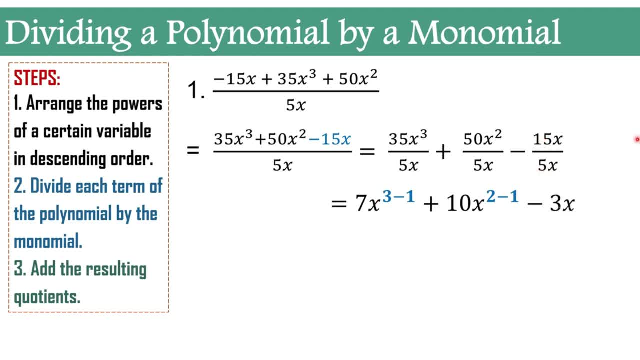 over 5. so 15 divided by 5, you will have negative 3 and for the exponent it will just be 1 minus 1. then after that you may simplify, subtract their exponent, so three minus one, that will become raised to two, and two minus one will become raised to one and one minus. 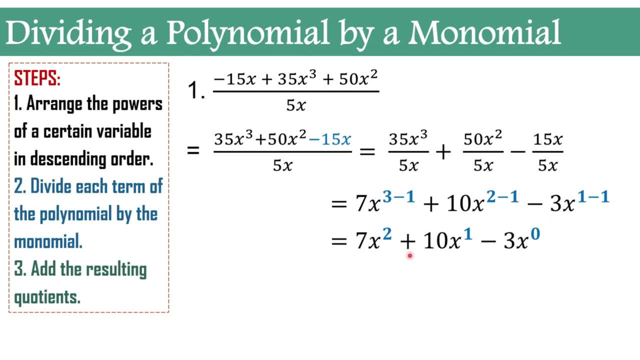 1 will become raised to 0.. But this is not yet the final answer. So this 7x squared. you may just copy that And then for positive 10x raised to 1, rule for exponent: you do not have to write it. 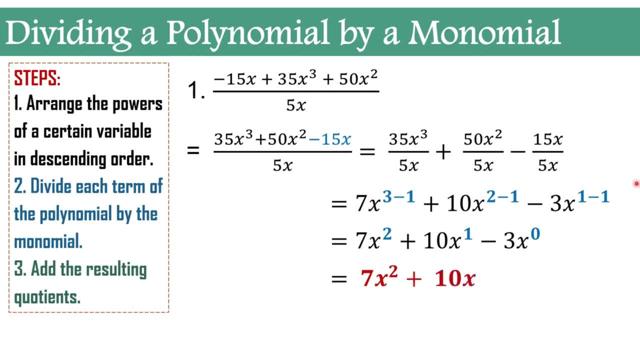 if the exponent is just 1.. So you will have positive 10x only. And then if the exponent of a variable is 0, automatically it will be equal to 1.. Any number raised to 0 is equal to 1.. So 1. 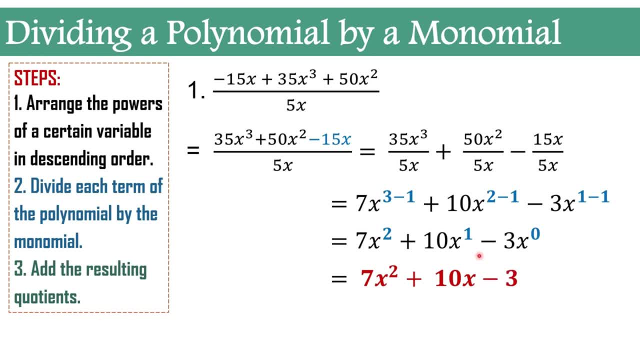 times 3, you will just have 3.. So your final answer will be 7x squared plus 10x minus 3.. Another example: 28p raised to 5 plus 21p cubed over 7p squared. Following the steps, 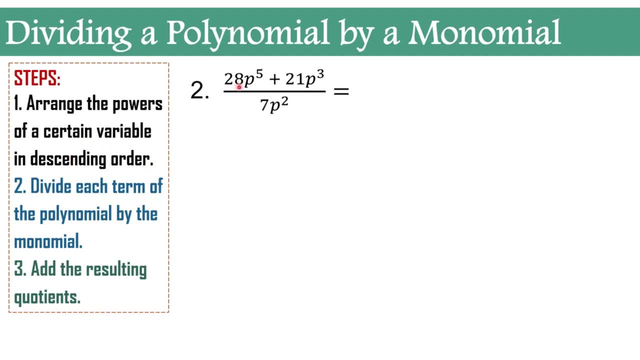 arrange the powers of a certain variable in descending order. As you can see, it's already arranged. So we're done with that. Let's proceed with the second step, which is dividing each term of the polynomial by the monomial. So it will be. 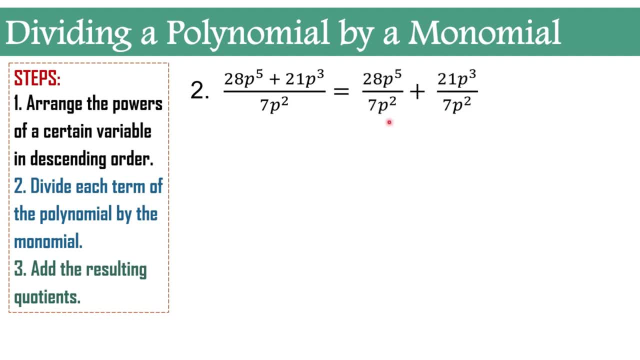 like this: 28p raised to 5 over 7p squared, plus 21p cubed over 7p squared. Let's start with 28 divided by 7.. So 28 divided by 7, you will have 4.. And for their variable, just subtract them. 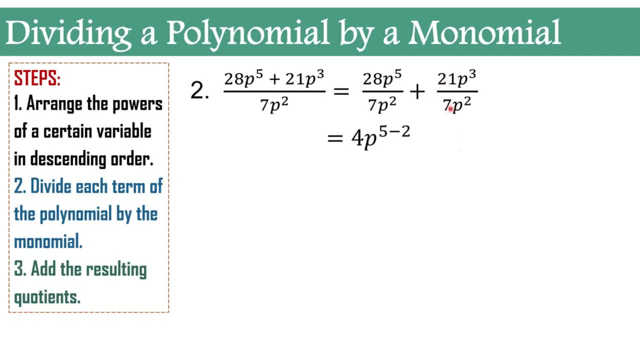 it will become 5 minus 2.. And then next, 21 divided by 7, you will have 3.. And p cubed divided by p squared, that will be 3 minus 2.. So simplify 4p and then 5 minus 2 is 3.. 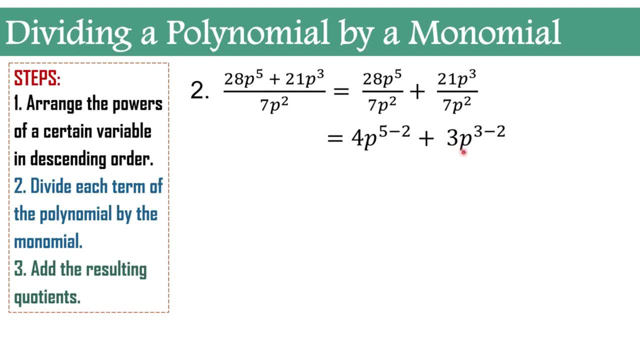 So you'll have 4p cubed, while 3p raised to 3 minus 2, that will be raised to 1.. So your final answer will become 4p cubed like this, and then plus 3p. The answer here is 1. And we do not have 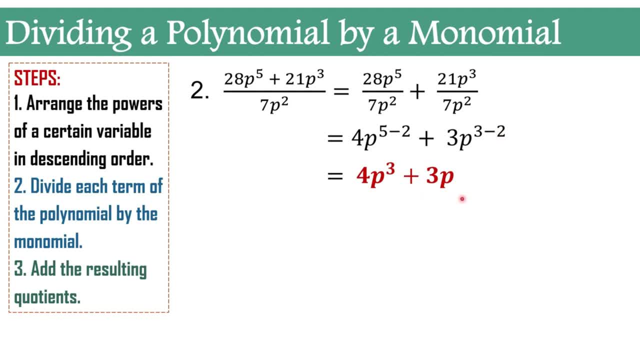 1 for the exponent. So we only have 3p. So the final answer is 4p cubed plus 3p. Another example: 15a squared b squared minus 27a squared b minus 3ab, divided by negative 3ab. 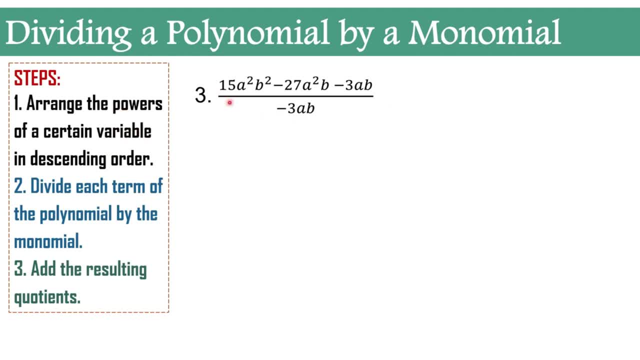 Again, first thing that you have to do is arrange the powers. As you can see, it's already arranged. So we have here 4, the sum of their exponent. we have here 3, and then 2.. Now we may proceed with the second step, which is dividing each term. 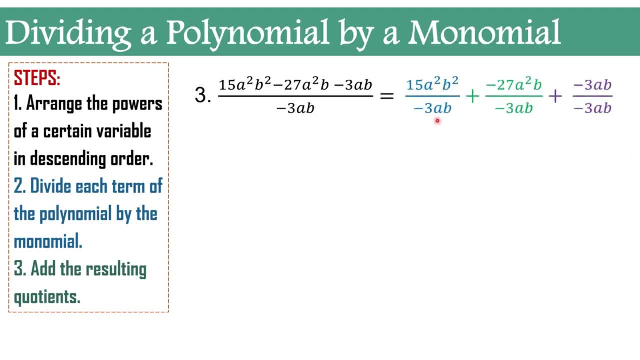 of the polynomial by the monomial given. So every term will have the denominator of negative 3ab. Let's proceed in dividing them: 15 divided by negative 3,. since the divisor is negative, your answer will be negative 5.. And then, for the variable, just subtract their exponent, So 2 and 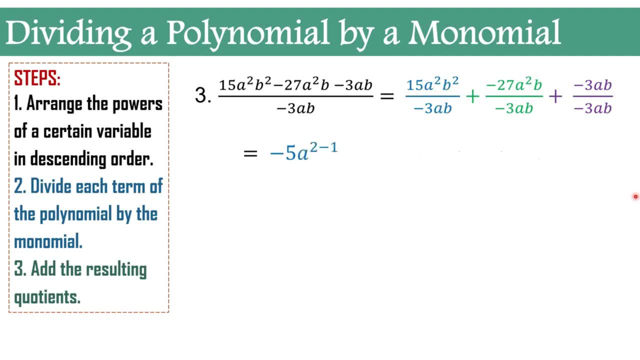 then raised to 1,, 2 raised to 1, that will be 2 minus 1.. For a and 2 minus 1, also for b. Then for the second term, negative 27 divided by negative 3, since both of them are negative, your answer will become positive, So we'll have positive 9.. 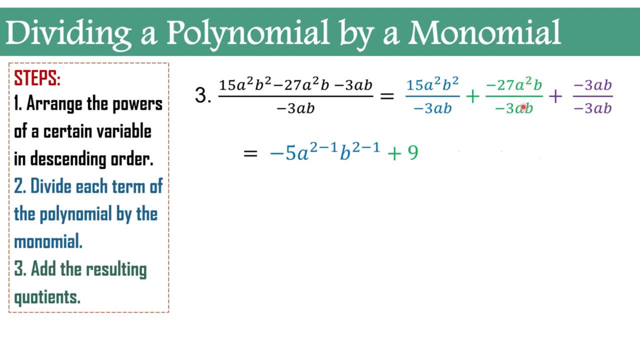 And then for the variable a, we have 2 and raised to 1, so 2 minus 1.. And for b, we have raised to 1, that will be 1 minus 1.. So for the last term, as you can see the numerator. 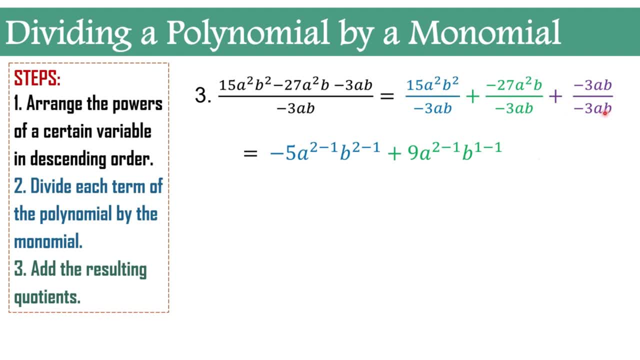 is exactly the same. So we have 2 and raised to 1, that will be 1 minus 1.. And then for the second term, the denominator is exactly the same. So we are dividing exactly the same term. So negative 3ab. 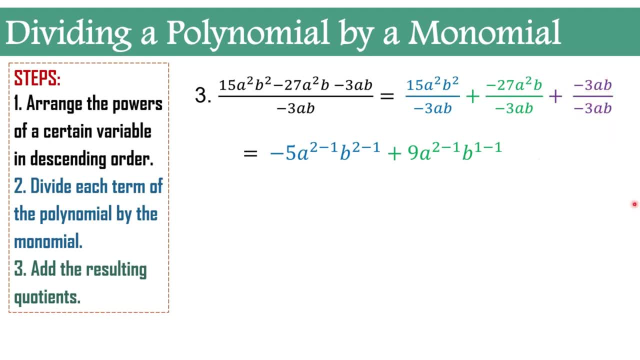 over negative 3ab, you will just have positive 1.. Both are negative, so your answer will become positive. Dividing the same number, you will obtain 1 as your answer. So let's simplify. Let's subtract their exponent For the first term, we'll have negative 3ab. 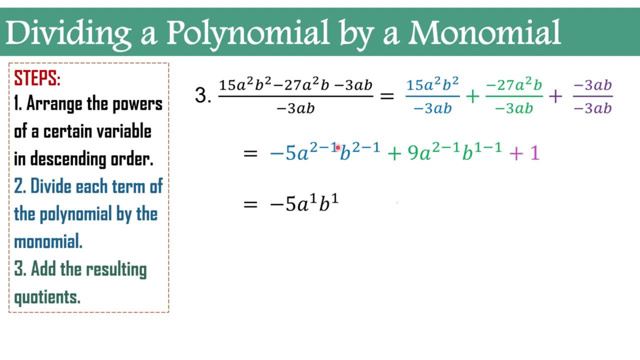 and then a raised to 1, and b raised to 1,, since 2 minus 1 is equal to 1.. For the second term, we have positive 9.. And a 2 minus 1,, you will have a raised to 1.. And 1 minus 1 for b. 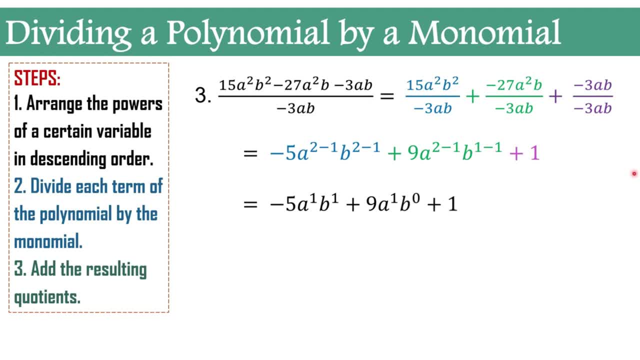 you will have b raised to 0. And copy the positive 1.. Now, since we do not have to write 1 as the exponent of the variable, we may just remove 1.. And then, for 0,, we will cancel out b. 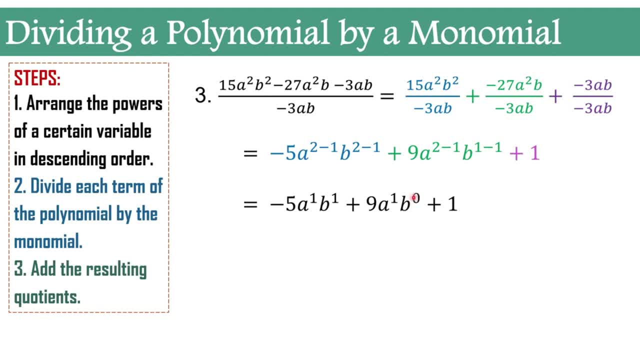 since b raised to 0 will just be equal, and when you multiply 1 to 9, you will still be getting 9.. So your answer will be negative: 5ab plus 9a. b raised to 0 is cancelled And then followed by the positive 1.. So the final answer. 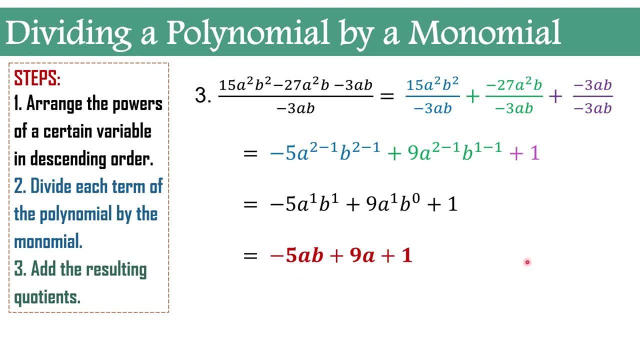 is negative: 5ab plus 9a plus 1.. Another example: 36x raised to 7, y raised to 5, minus 12x raised to 4, y raised to 6.. All over 12x squared, y cubed. So again, arrange this first And, as you can see, 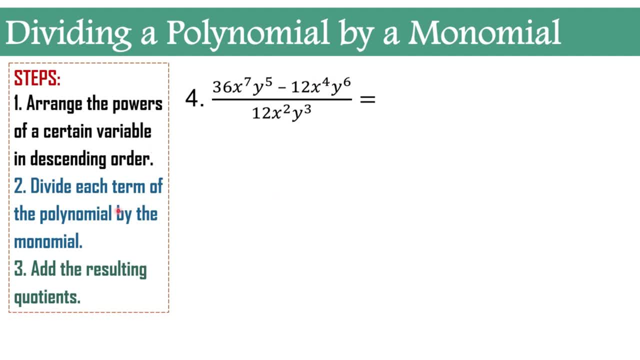 it's already arranged. So we're done with the step 1.. Now let's proceed with the second step, which is dividing them by the monomial in the denominator. So it will be like this, And when you divide, you may start with the numerical coefficient 36 divided by 12,. 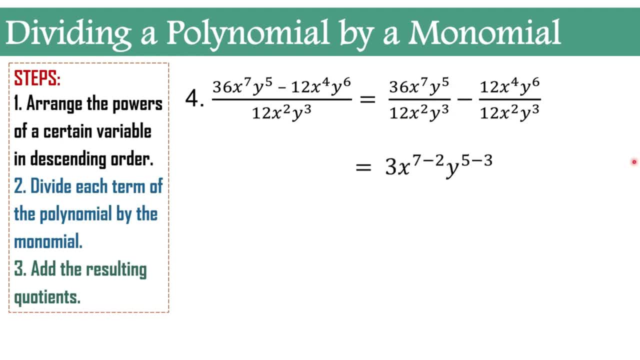 followed by their variables. So 36 divided by 12, you will have 3.. And then for the variable it will become 7 minus 2 for x, and then 5 minus 3 for y, And for the next term, 12 divided by 12,. 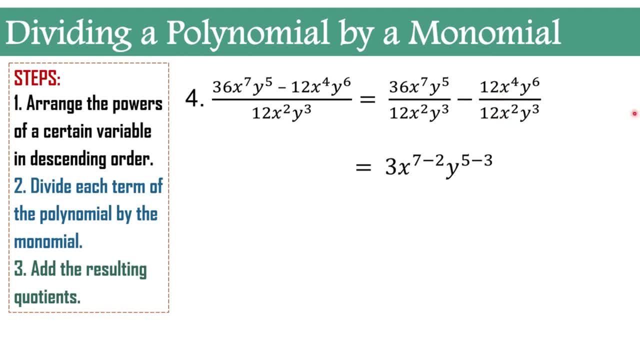 you will just get 1.. And then for the variable, just subtract their exponent. So now let's proceed in subtracting their exponent. Just copy the numerical coefficient 3, and subtract 7 minus 2 and 5 minus 3.. You will have x raised to 5, and then y raised to 2.. And for the 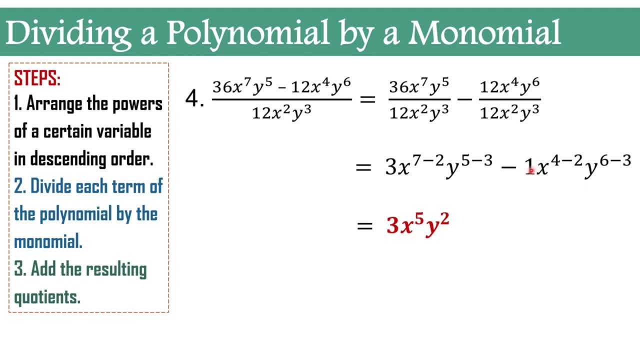 last term. since the numerical coefficient is 1, you may not write it. Okay, We are not writing 1 as the numerical coefficient, So we may proceed with the variable subtracting 4 minus 2 and 6 minus 3 for y. So we'll have negative x squared and y cubed. So the final answer is 3x raised to. 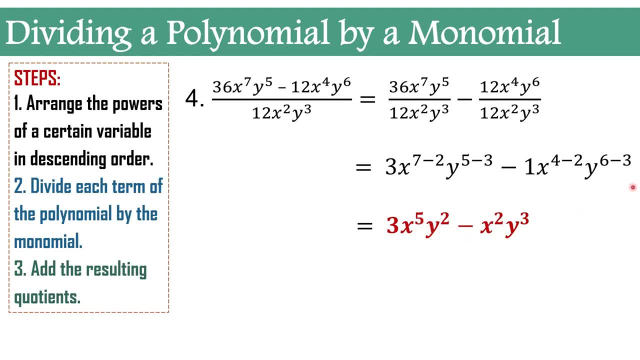 5y squared minus x squared y cubed. Okay, Next example: negative 6m squared plus 8, all over 12m. So for the first step, arrange the powers of a certain variable in descending order. As you can see, it's not arranged, So we must write 9m cubed first, before negative 6m. 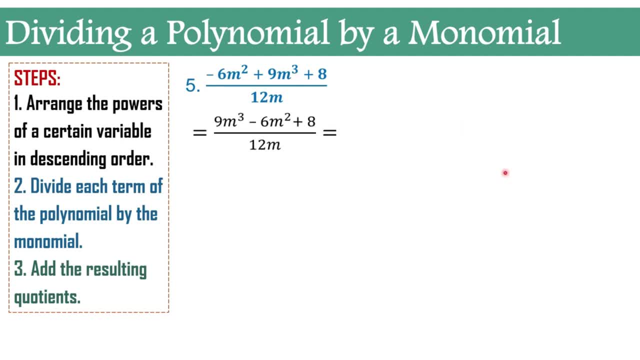 squared. Since 3 is the highest exponent, it will become like this: 9m cubed minus 6m squared plus 8.. So we're done with the first step. Let's proceed with the second step by dividing each term by 12m. So we have now 9m cubed divided by 12m. So let's divide their numerical coefficient. 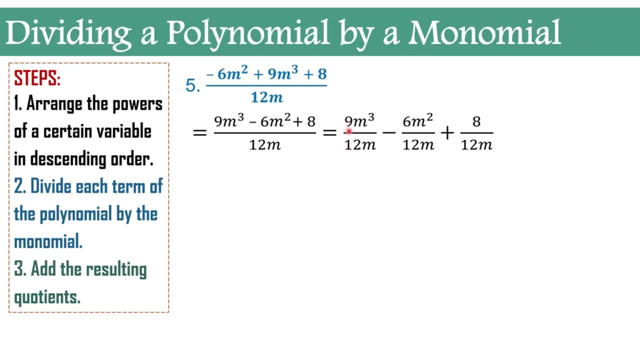 Actually you cannot divide them. You may just simplify them. So imagine the fraction 9 over 12.. Simplify That, will become 3 over 4.. And then for the variable, just subtract them. You will have 3 minus 1, since 3 is the exponent of the variable in the numerator and 1 for the denominator. 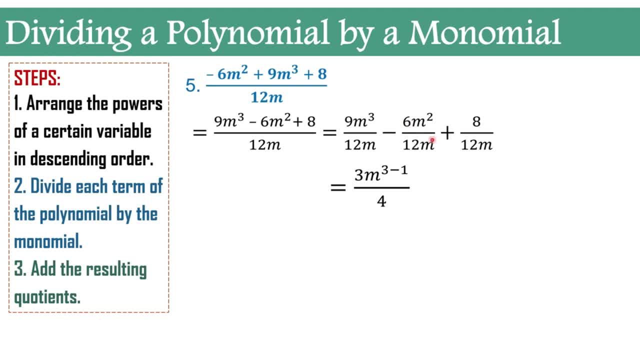 Second term. so 6 over 12, when you simplify that will become 1: half And the numerical coefficient 1, we do not have to write it. Okay, 1 here, but we did not write it anymore, since we. 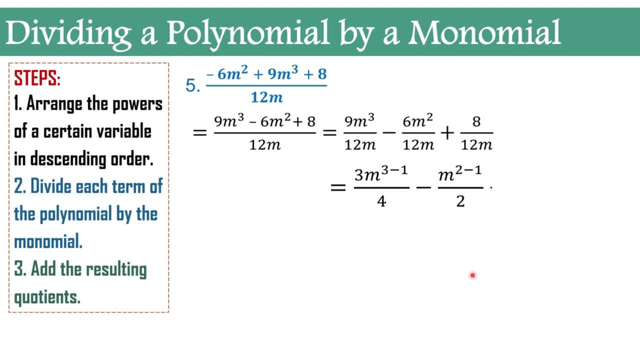 do not write 1 if it is numerical coefficient. So for the variable we just have to divide m squared and m. You will have 2 minus 1.. And for the last term, 8 over 12.. So 8 over 12,. 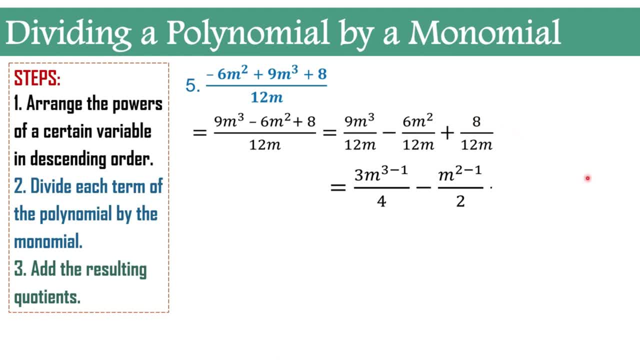 just simplify and copy the variable m- 8 over 12 will become 2 over 3- and copy the variable m, Then simplify, So simplifying their exponent. you just have to subtract and then copy the rest, So you'll have 3m raised to 2, since 3 minus 1 is 2, over 4, followed by m, 2 minus 1 will become 1.. 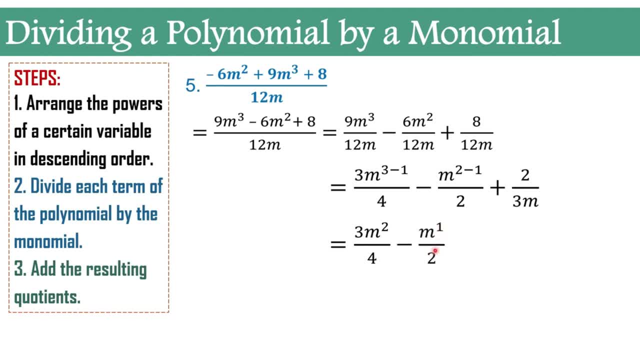 So you will just have negative m raised to 1 over 2.. And for the last term, just copy it. Okay? And then this is not yet the final answer. since you can see 1 as the exponent of m, We may just remove this, because we do not have to write 1 if it is an exponent. So your 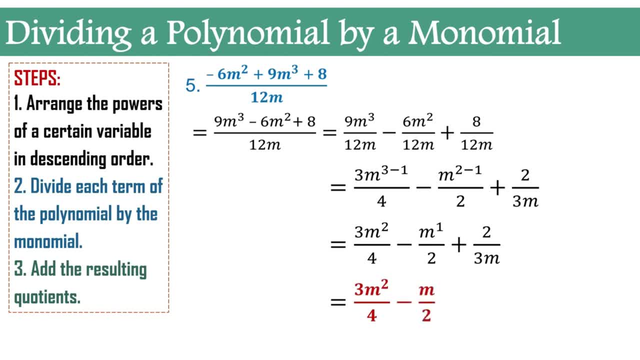 answer will be 3m squared over 4 minus m over 2.. We remove 1 plus 2 over 3m. Okay, And for the last example, we have 8 over 12.. So we do not have to write 1 if it is an exponent. So your answer will be: